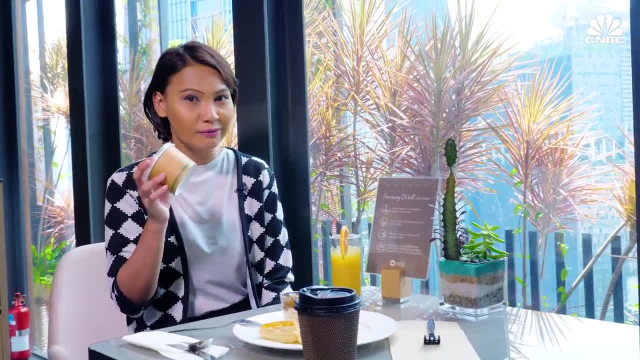 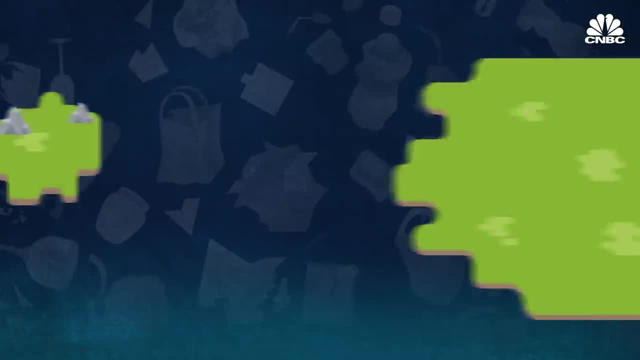 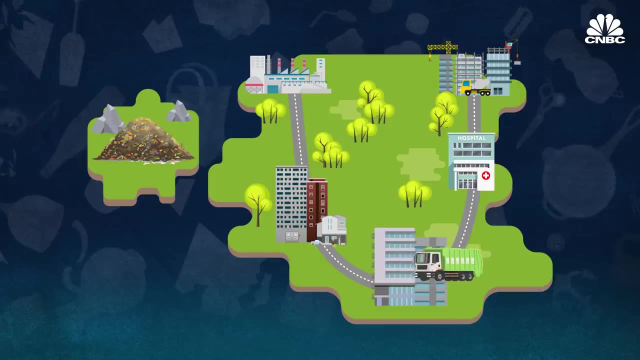 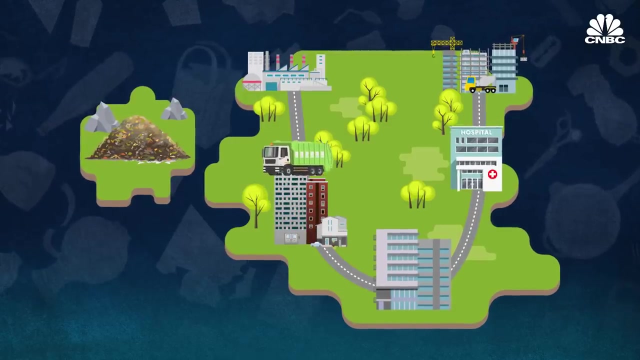 can keep pace with this growing problem. So what's the solution? The waste management process comprises the collection, treatment and disposal of waste. Solid waste can come from several sources, mainly from residential and commercial properties and industrial facilities such as medical, electronic and construction waste. 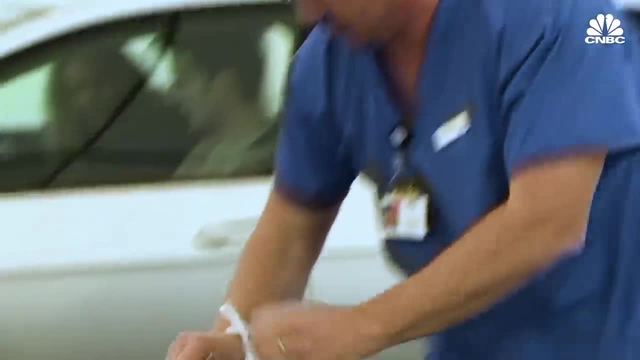 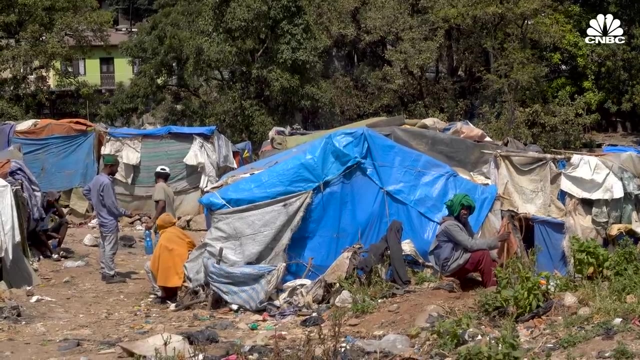 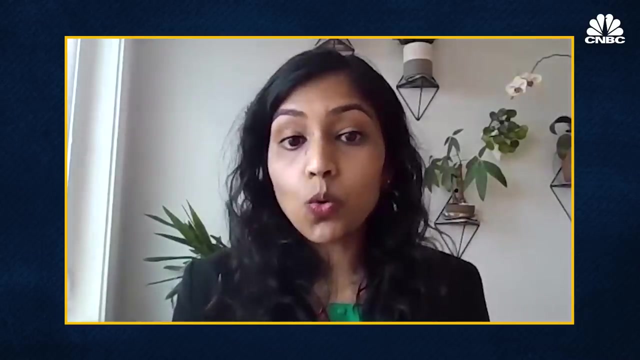 With COVID. overall, we've seen medical waste increase about 40%. It's often the poor that are the most affected by lack of waste management services, whether it's because they're not receiving waste management services due to where they're living, or waste is being dumped by the communities. 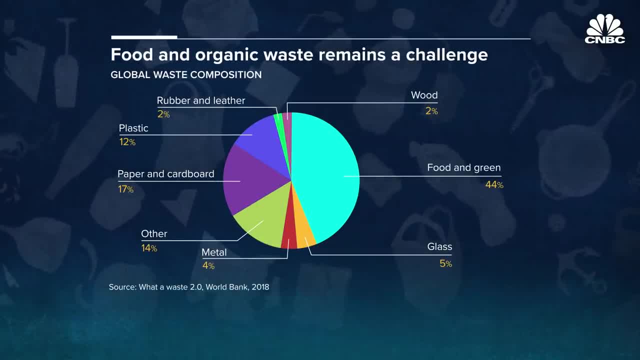 Even as medical waste piles up, it's a tiny fraction of municipal solid waste. Of the 2 billion tonnes of waste generated globally, 12% is plastic waste, but it's dwarfed by food and organic matter and paper and cardboard scraps. 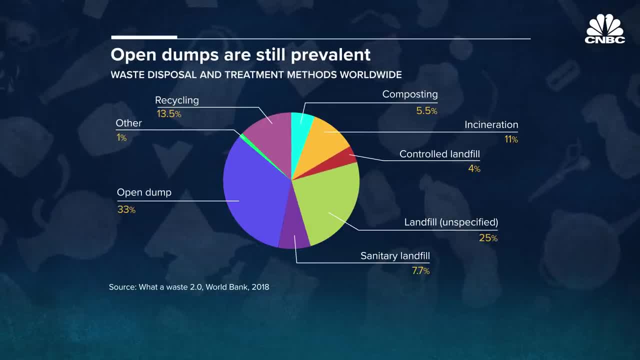 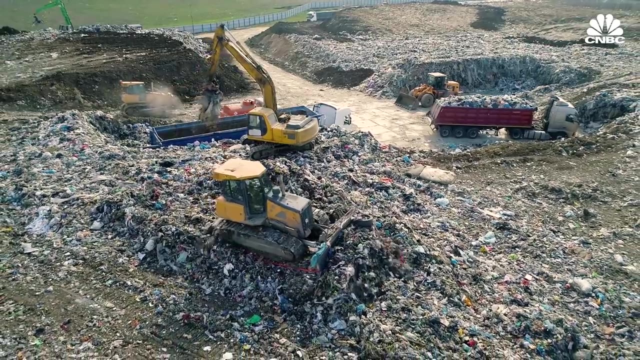 Once all that trash is collected, there are three main ways it is treated and disposed of: by burning the trash in an incinerator, using a landfill or dumping it openly without any processing whatsoever, While 33% of global waste end up directly at open dumps. 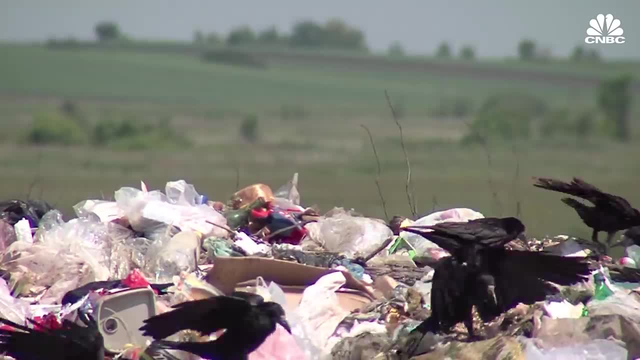 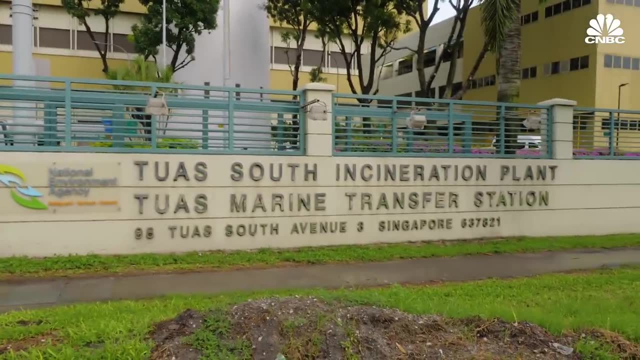 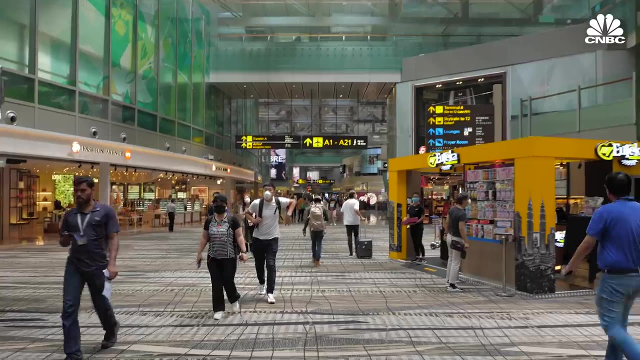 governments are increasingly recognising that these sites are bad for the environment and can be vectors for diseases. Instead, they are opting for more sustainable ways to manage their waste, such as incinerators and recycling programmes. Nowhere is this more pronounced than in densely populated Singapore. 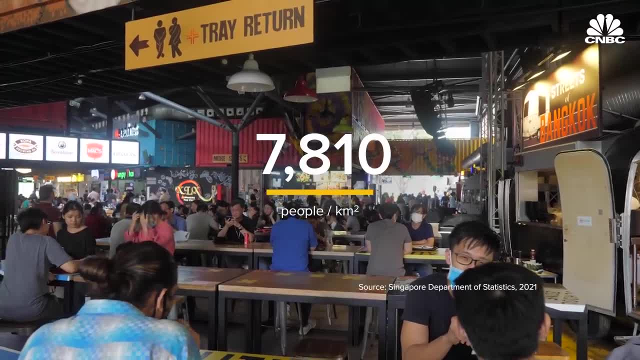 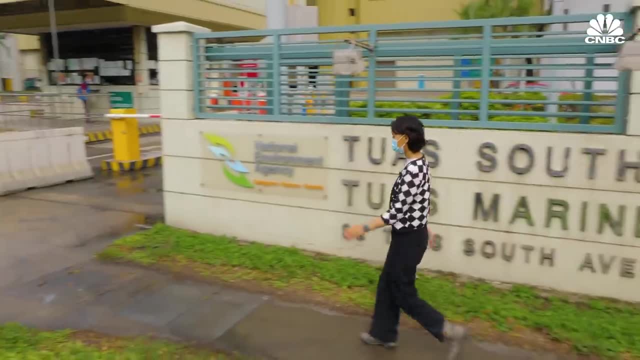 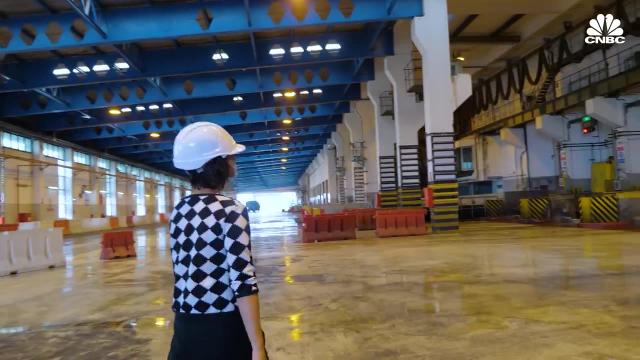 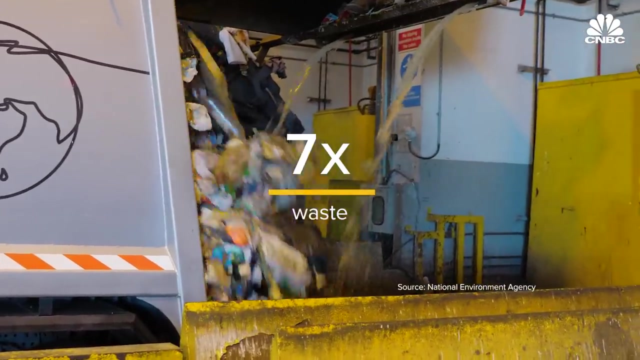 which has nearly 8,000 people per square kilometre, more than 17 times that of India and 200 times that of the US. Between 1970 and 2016,, the amount of solid waste disposed in Singapore increased about sevenfold as its population and economy grew. 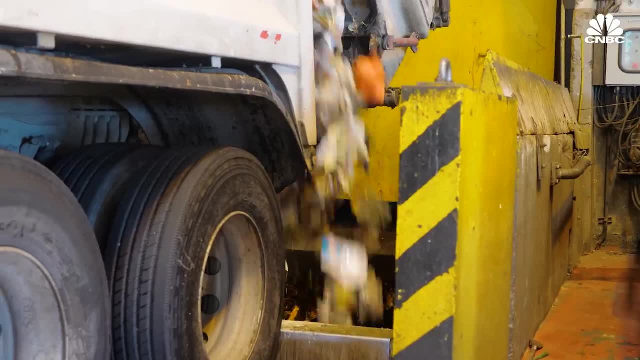 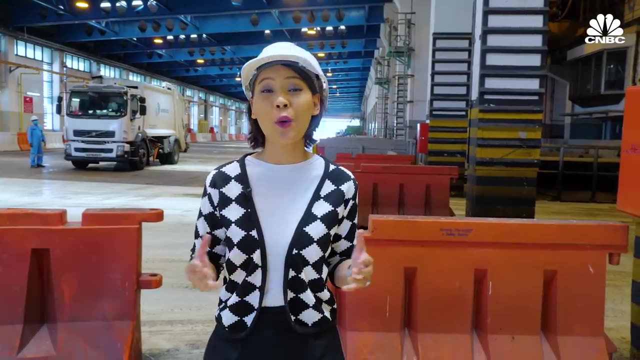 Of the 7 million tonnes of waste generated in the country in 2019, more than half were recycled. The journey of a single piece of trash brings us to Tuas South Incineration Plant, the largest waste incineration facility in Singapore to date. 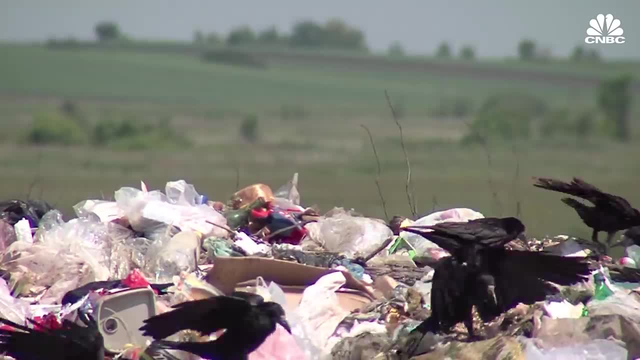 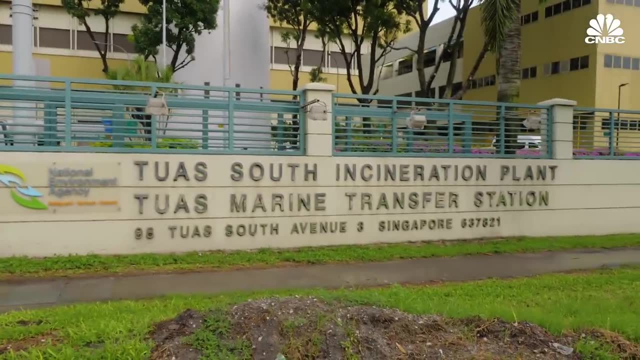 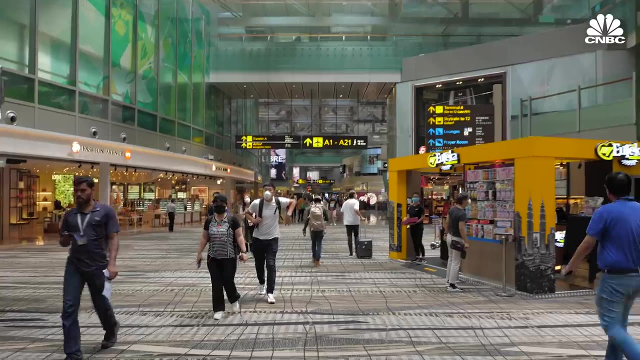 governments are increasingly recognising that these sites are bad for the environment and can be vectors for diseases. Instead, they are opting for more sustainable ways to manage their waste, such as incinerators and recycling programmes. Nowhere is this more pronounced than in densely populated Singapore. 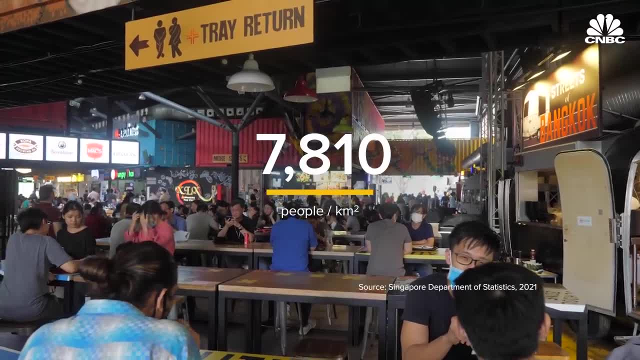 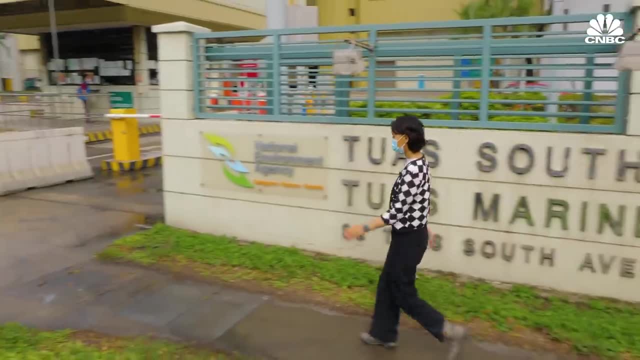 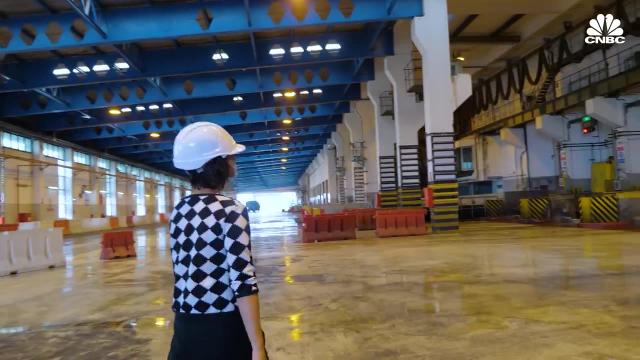 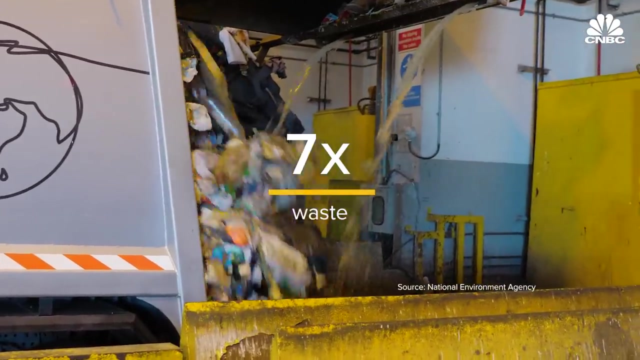 which has nearly 8,000 people per square kilometre, more than 17 times that of India and 200 times that of the US. Between 1970 and 2016,, the amount of solid waste disposed in Singapore increased about sevenfold as its population and economy grew. 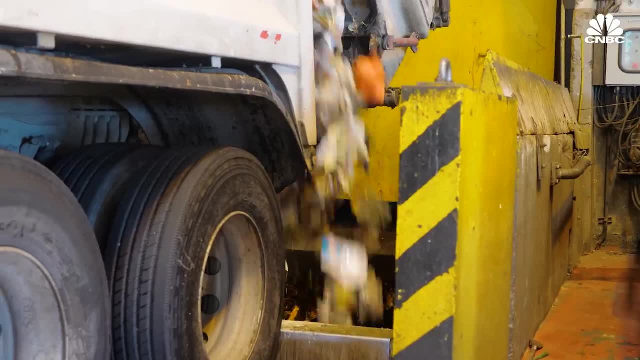 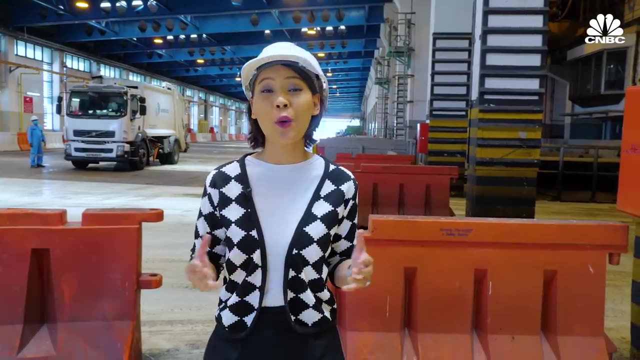 Of the 7 million tonnes of waste generated in the country in 2019, more than half were recycled. The journey of a single piece of trash brings us to Tuas South Incineration Plant, the largest waste incineration facility in Singapore to date. 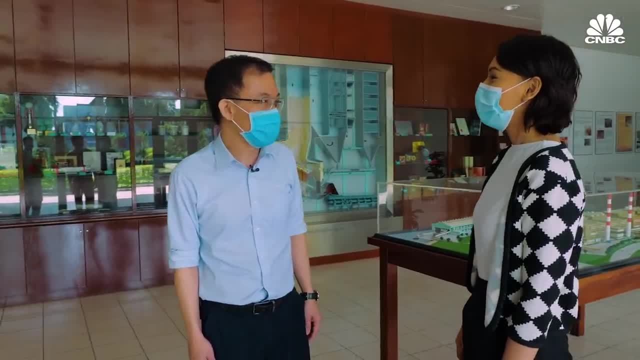 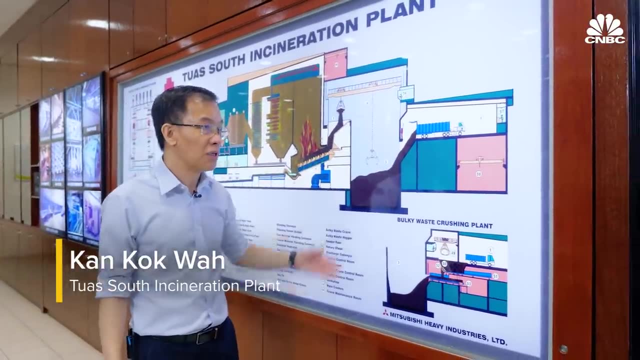 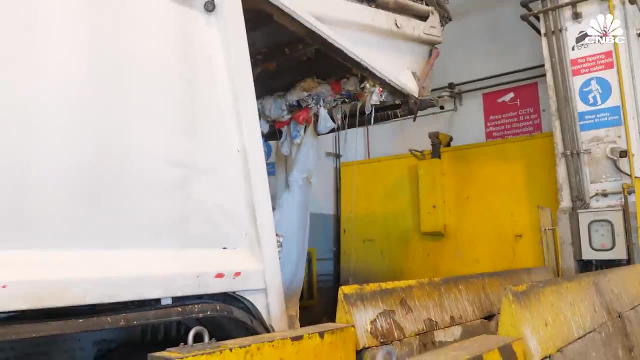 Kan Kok Wah is the general manager of the plant, one of four such facilities in the country which can convert waste into energy. Waste is collected from the industrial, commercial premises and household premises. The average of about 600 trucks are coming to Tuas South Incineration Plant. 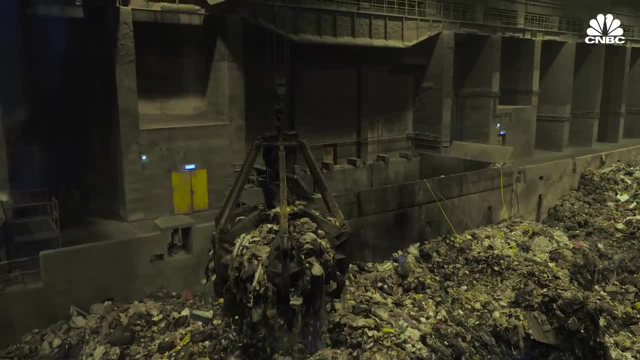 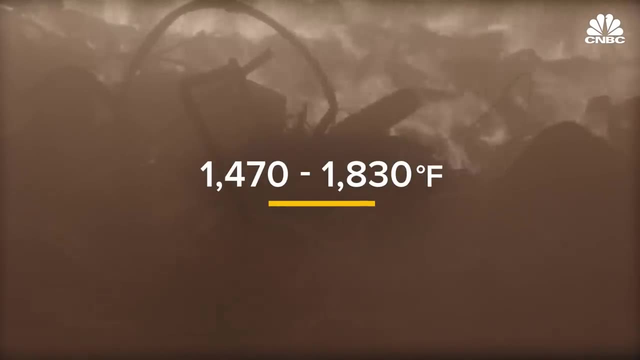 They will discharge the waste into the bunker. Cranes will then grab and feed the waste into the incinerator. The furniture in the furnace is about 850 to 1,000 degrees. It will achieve a 90% reduction in terms of volume. 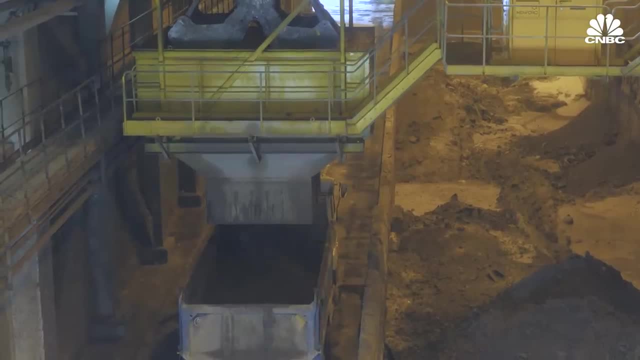 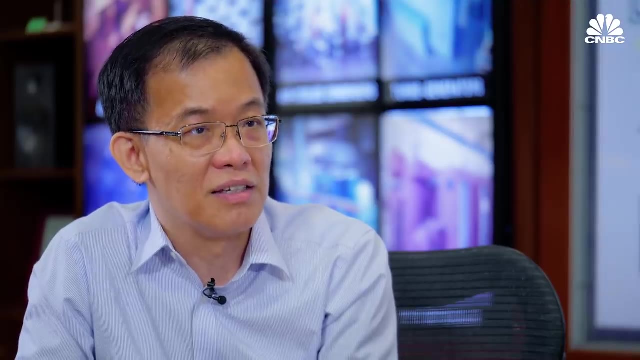 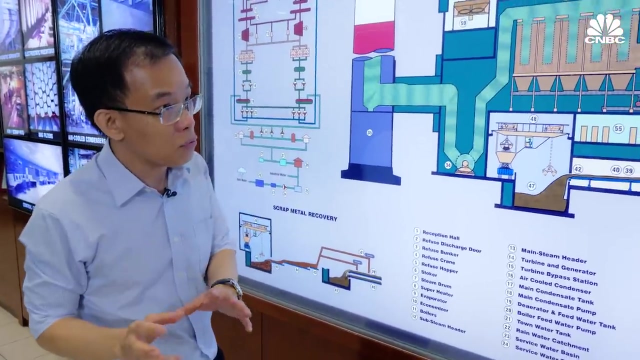 This will then help to conserve the space required for landfill. Singapore is a very small country. It's land scarce, so the need to conserve land is very critical for Singapore. Along the way, we have magnetic separator. Furious and non-furious matter will be recovered from the ash. 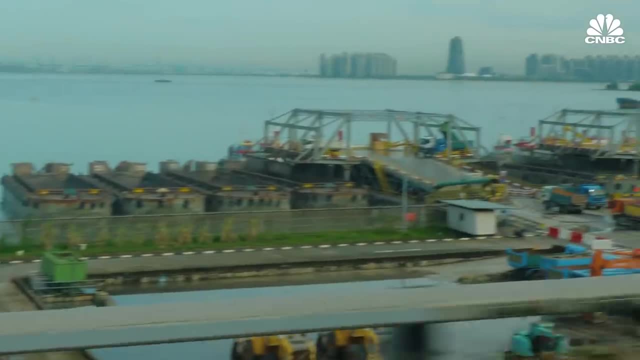 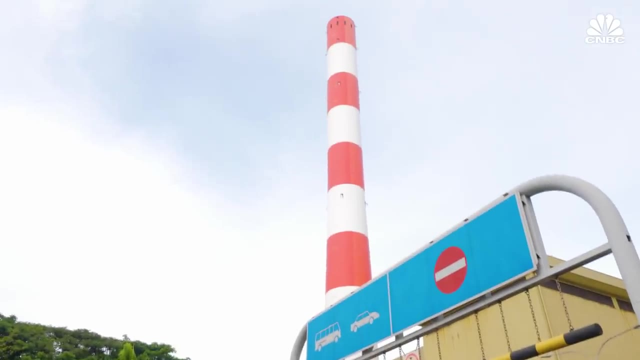 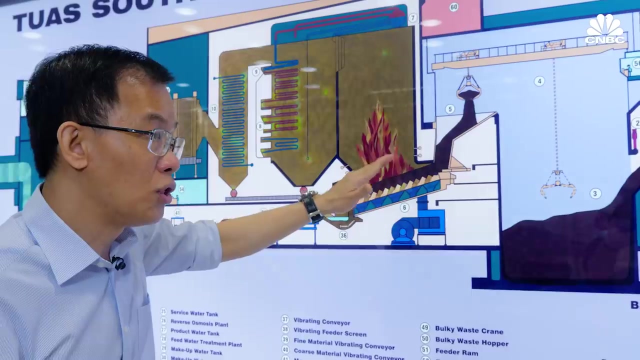 Ash will then be transported from the ash pit to another facility. Pollutants produced during incineration are treated before being released into the atmosphere, ensuring clean air is being discharged. Water will be converted into steam From the energy recovery. it will be recovered from the combustion of waste. 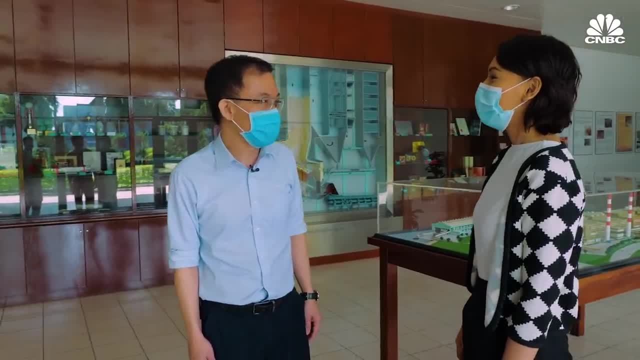 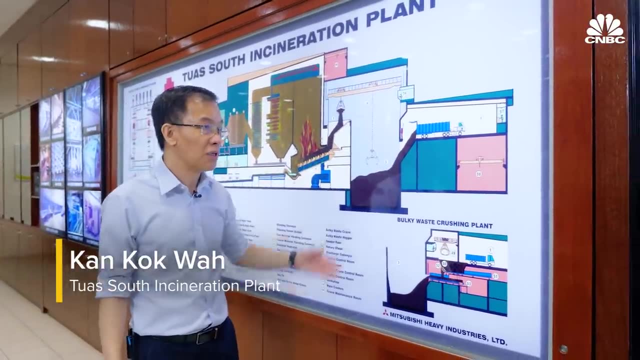 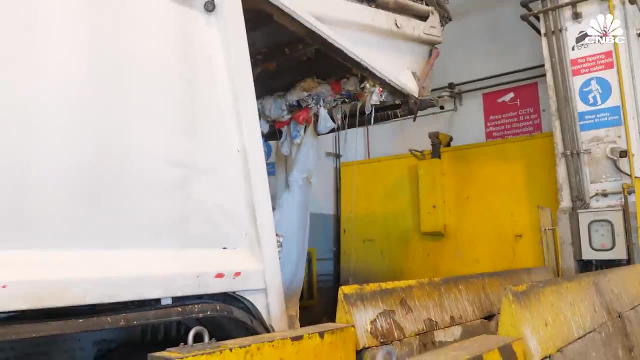 Kan Kok Wah is the general manager of the plant, one of four such facilities in the country which can convert waste into energy. Waste is collected from the industrial, commercial premises and household premises. The average of about 600 trucks are coming to Tuas South Incineration Plant. 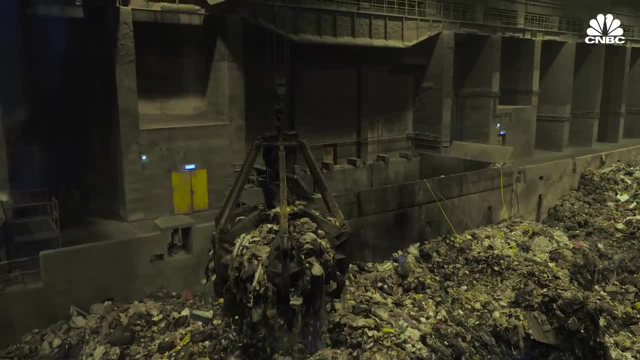 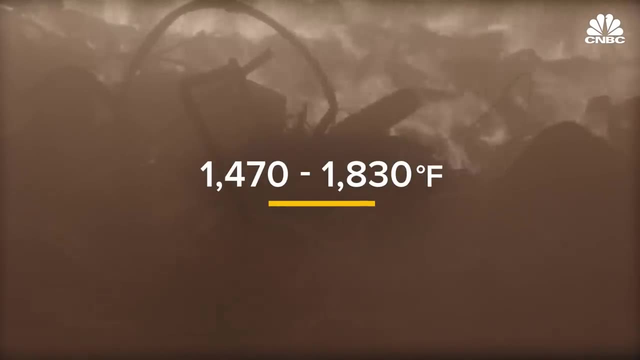 They will discharge the waste into the bunker. Cranes will then grab and feed the waste into the incinerator. The furniture in the furnace is about 850 to 1,000 degrees. It will achieve a 90% reduction in terms of volume. 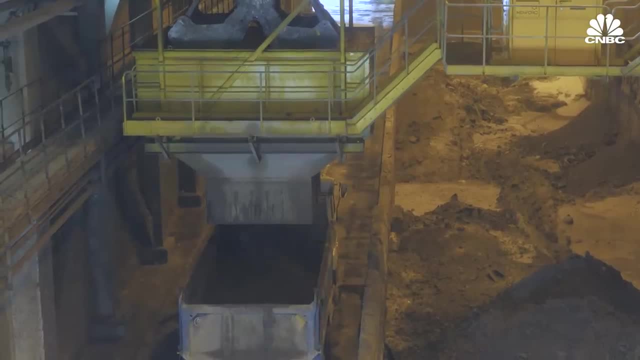 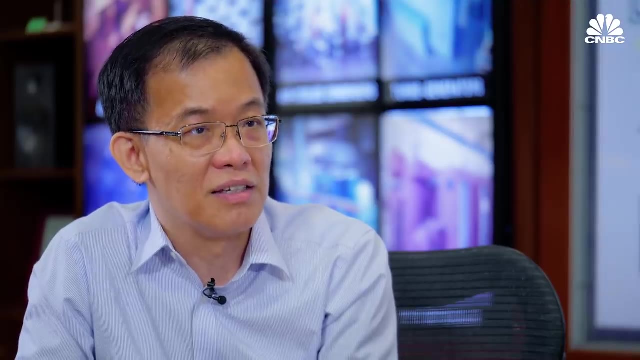 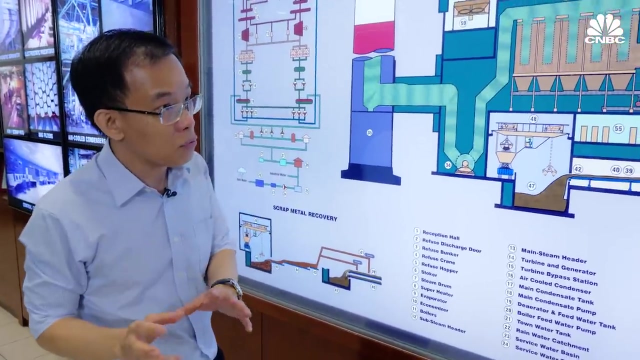 This will then help to conserve the space required for landfill. Singapore is a very small country. It's land scarce, so the need to conserve land is very critical for Singapore. Along the way, we have magnetic separator. Furious and non-furious matter will be recovered from the ash. 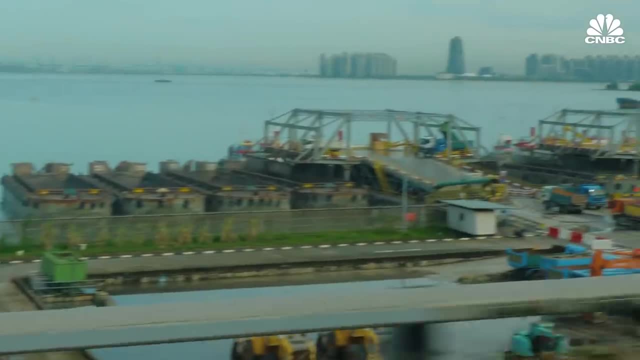 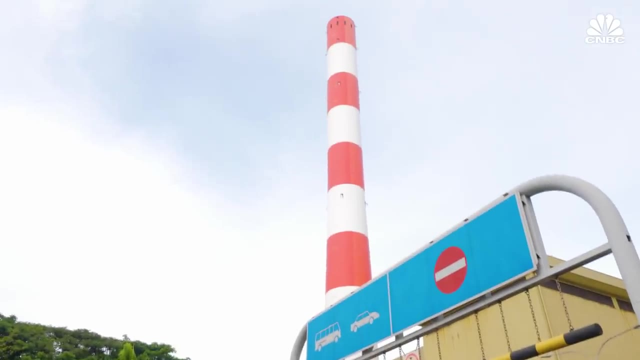 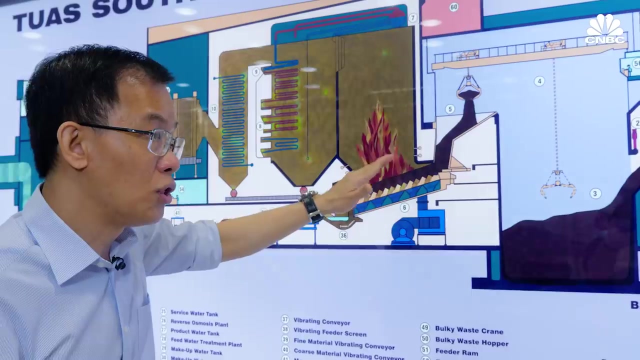 Ash will then be transported from the ash pit to another facility. Pollutants produced during incineration are treated before being released into the atmosphere, ensuring clean air is being discharged. Water will be converted into steam From the energy recovery. it will be recovered from the combustion of waste. 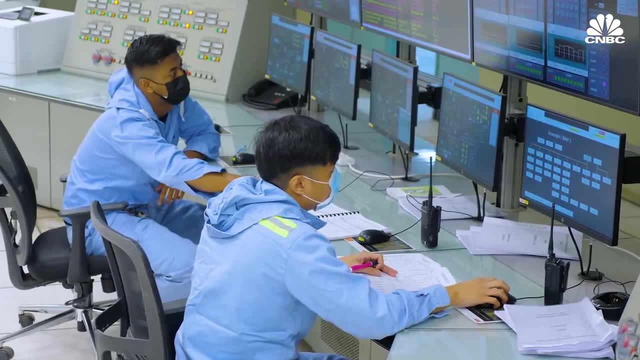 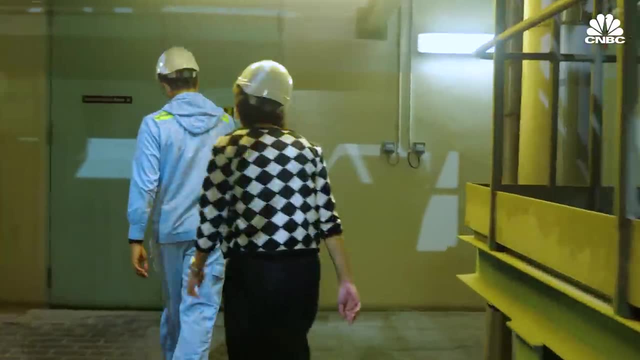 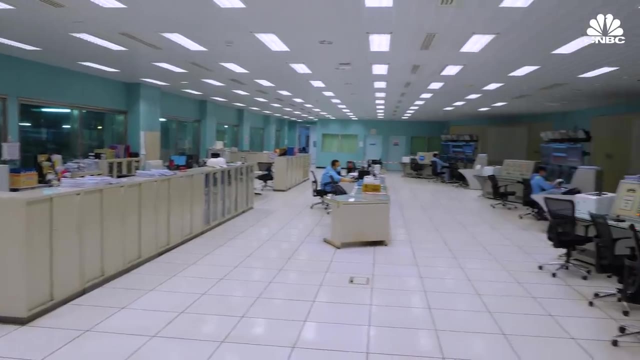 This water will be then converted into high-temperature, high-pressure steam to run turbine generators. This is to produce electricity power. 20% is being consumed internally, with the rest being exported to the national grid. The total power generated by the four waste-to-energy incineration plants in Singapore. 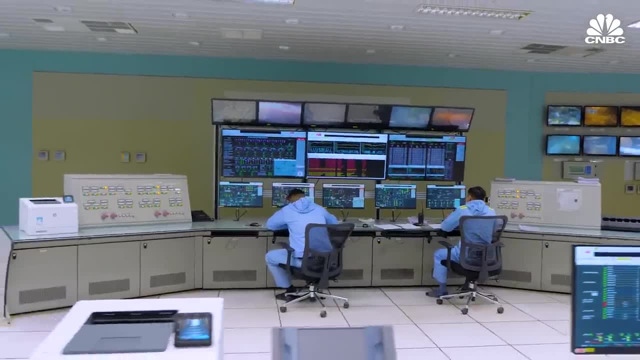 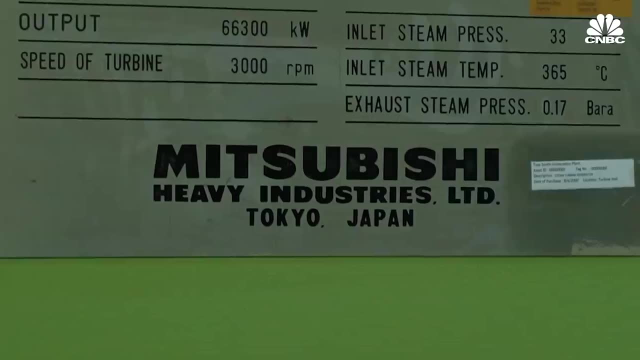 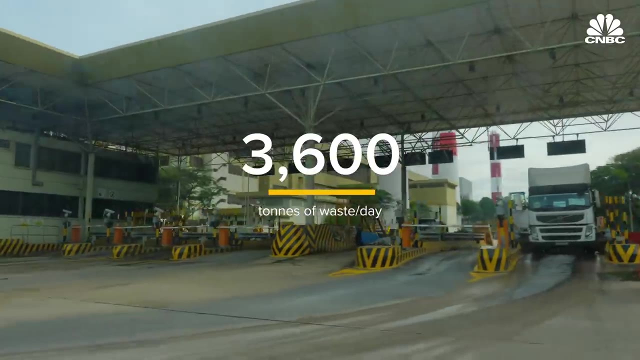 including Tuas South, contributes about 2 to 3% to the national electricity demand in the country. An upcoming waste-to-energy plant built by Mitsubishi Heavy Industries and water treatment company Hiflux will be able to incinerate 3,600 tonnes of waste per day. 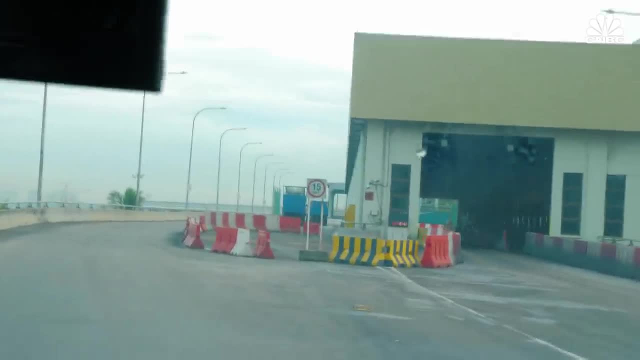 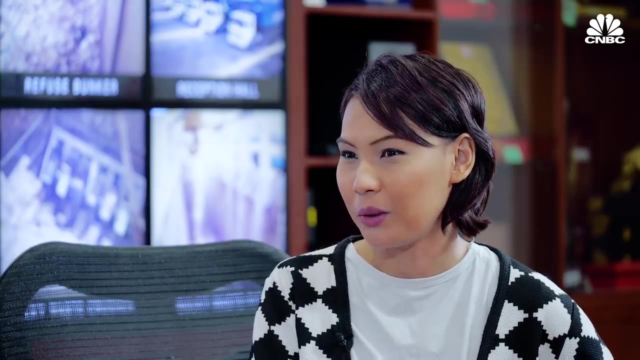 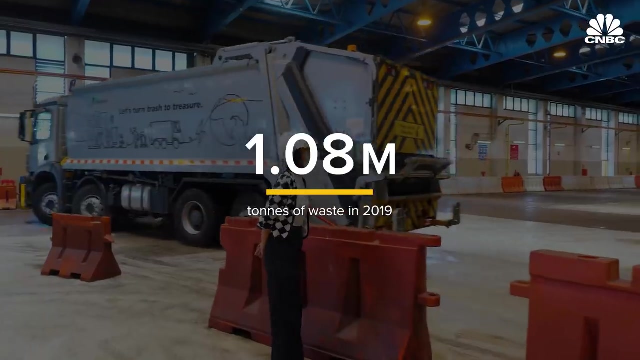 while generating electricity to be self-sufficient and providing access power to the national grid. How much waste is collected and managed in TSIP? In 2019, about 1.08 million tonnes of waste is collected. That's equivalent to about 3,000 tonnes of waste daily. 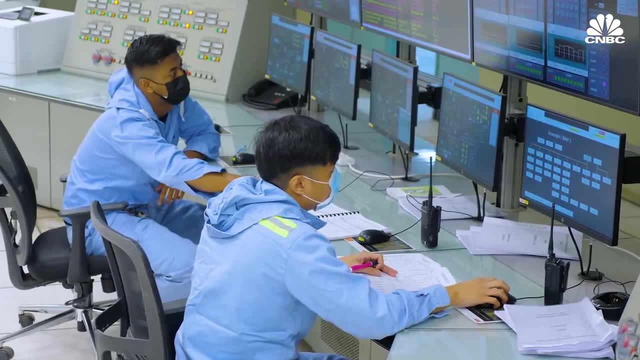 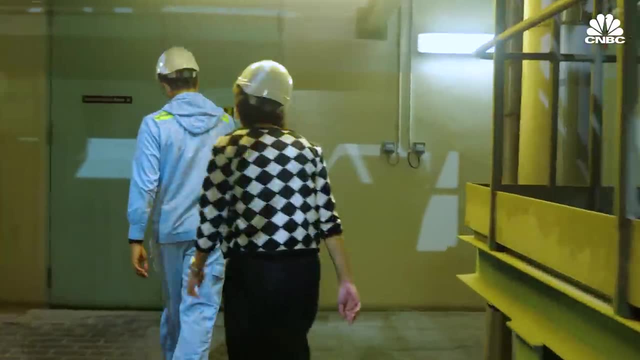 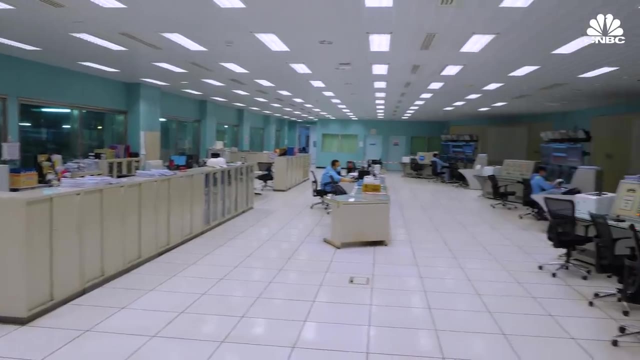 This water will be then converted into high-temperature, high-pressure steam to run turbine generators. This is to produce electricity power. 20% is being consumed internally, with the rest being exported to the national grid. The total power generated by the four waste-to-energy incineration plants in Singapore. 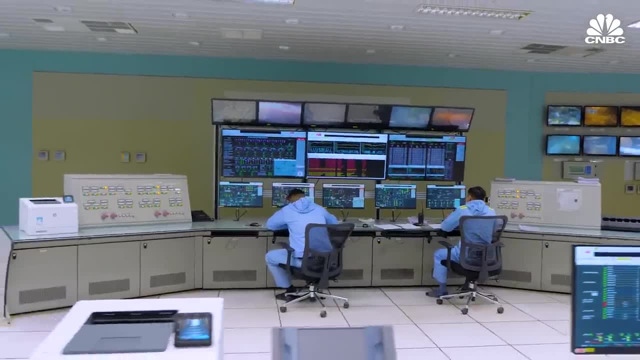 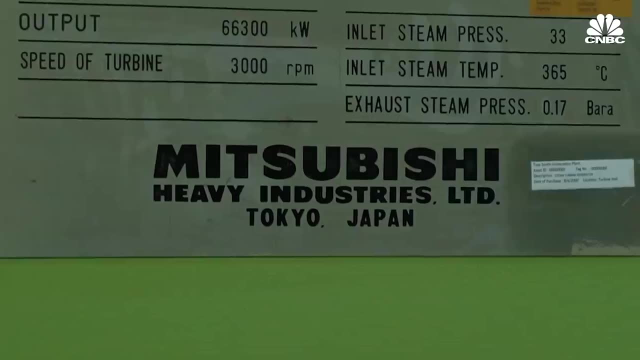 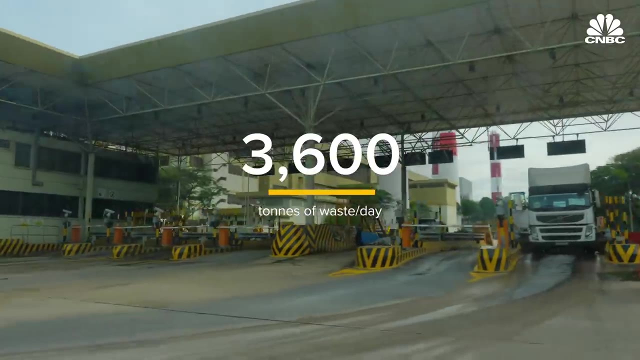 including Tuas South, contributes about 2 to 3% to the national electricity demand in the country. An upcoming waste-to-energy plant built by Mitsubishi Heavy Industries and water treatment company Hiflux will be able to incinerate 3,600 tonnes of waste per day. 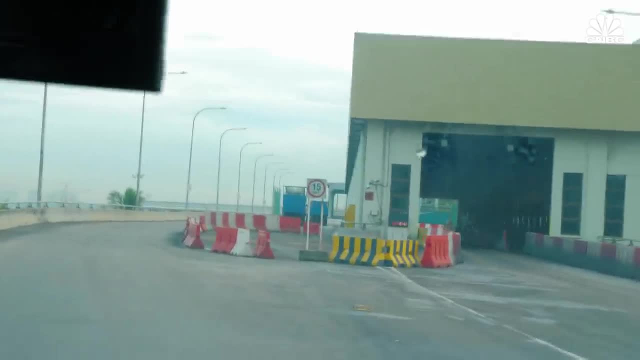 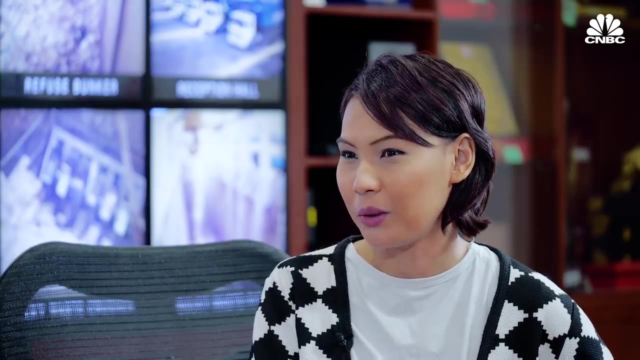 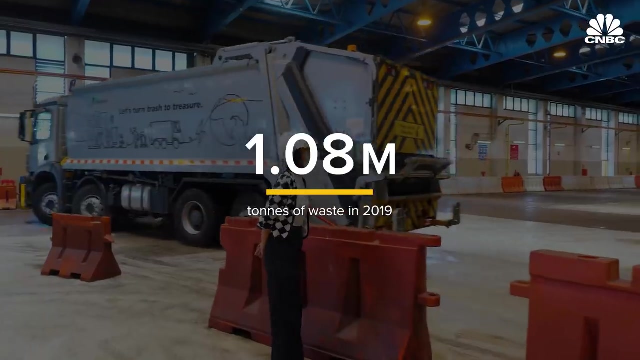 while generating electricity to be self-sufficient and providing access power to the national grid. How much waste is collected and managed in TSIP? In 2019, about 1.08 million tonnes of waste is collected. That's equivalent to about 3,000 tonnes of waste daily. 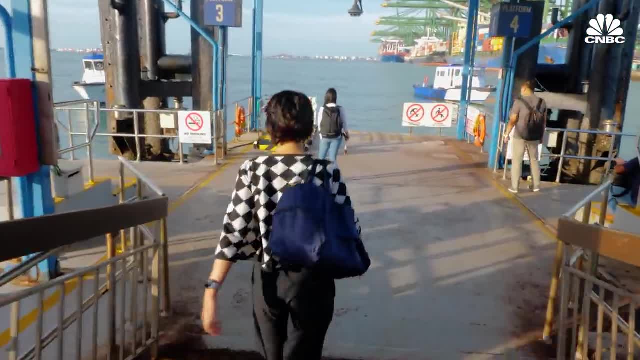 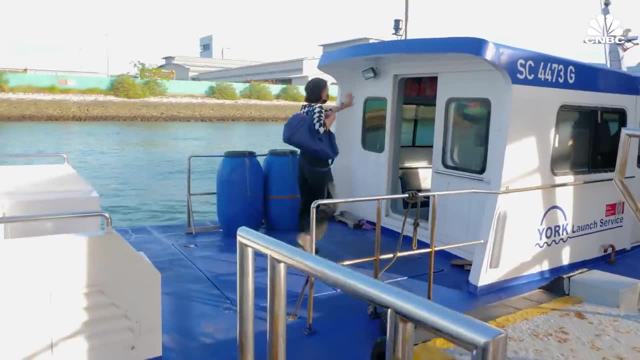 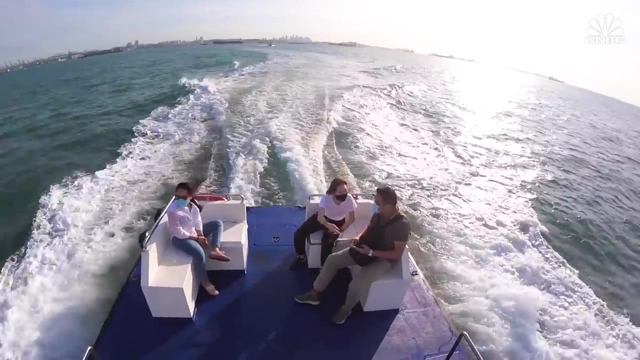 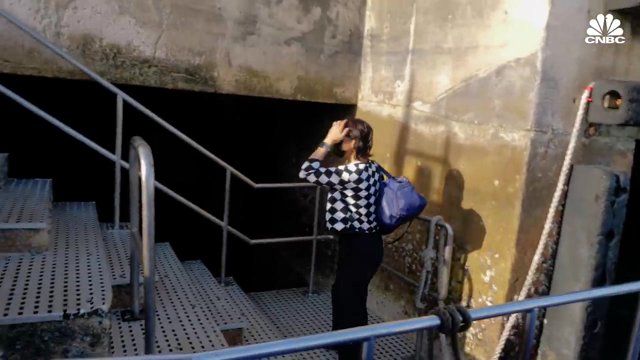 After the incineration process, my journey takes me on a ferry to the country's only landfill, located along the Singapore Strait, one of the busiest waterways in the world. The island's name is Samakau Landfill. Samakau Landfill is an offshore landfill. 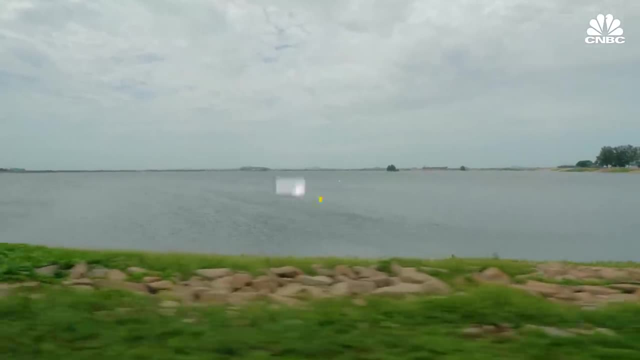 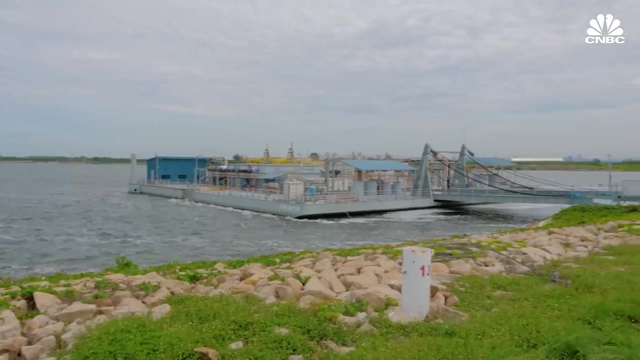 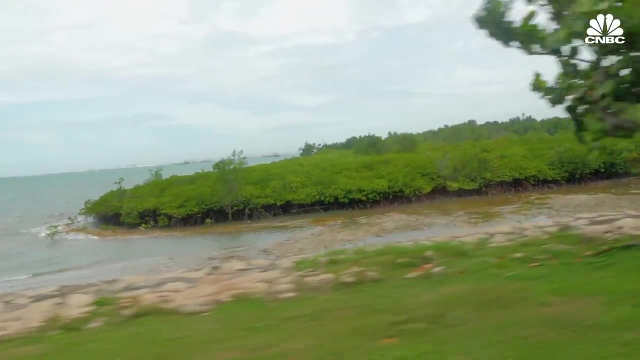 enclosed by a 4.3-mile perimeter rock embankment, which creates a sea space to fill with incinerated rubbish. In operation since 1999 and costing nearly half a billion dollars, the island is more than just a landfill. The island is more than just a landfill. 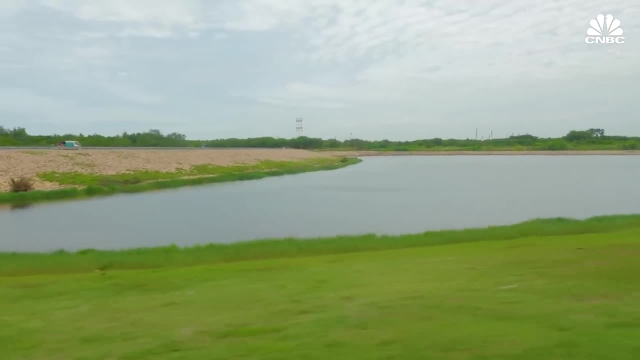 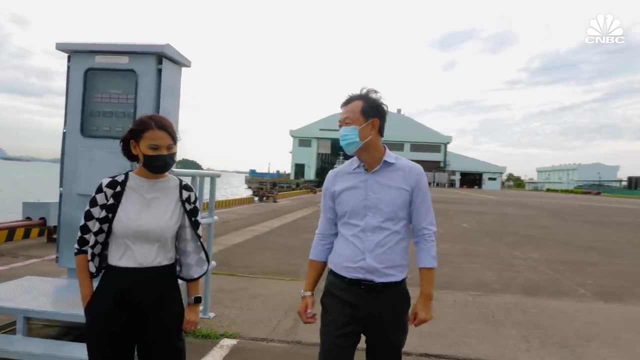 We make up of two big islands called the Pulau Samakau and Pulau Sake. These are two joined together into what we call what you see here: a 350 hectares Pulau Samakau Landfill, A barge ferries, more than 2,000 tonnes of waste. 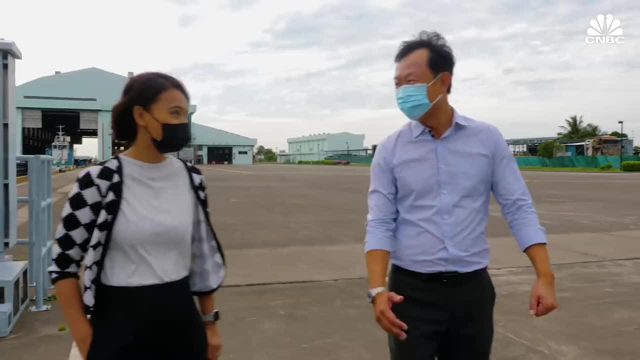 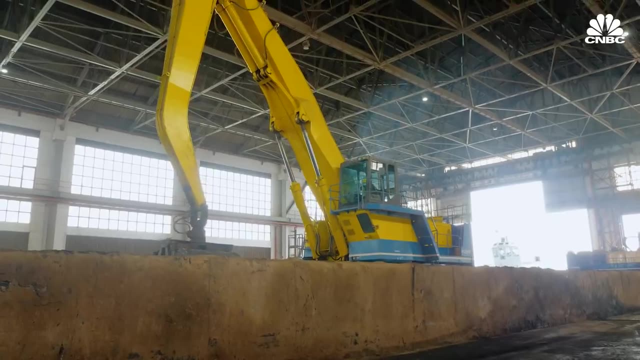 between mainland Singapore and Samakau Landfill daily, says Desmond Lee, General Manager of the landfill. We have big equipment such as the dump truck, excavators, etc. These are equipments that we use to collect waste. These are equipments that we use to collect waste. 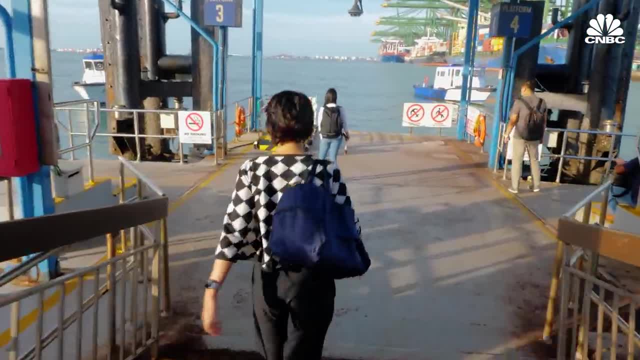 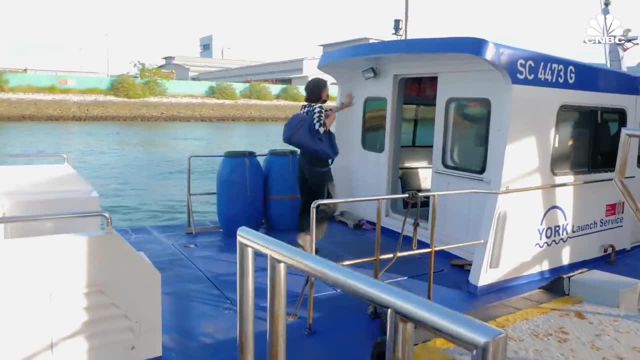 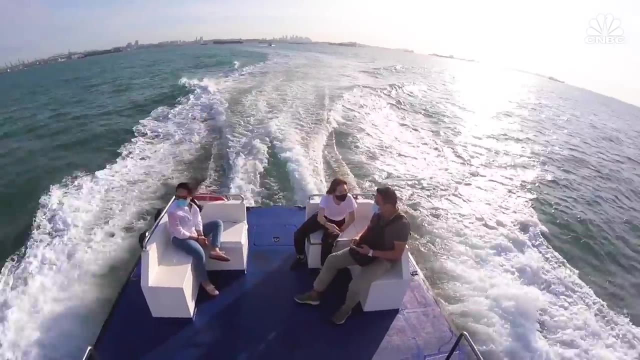 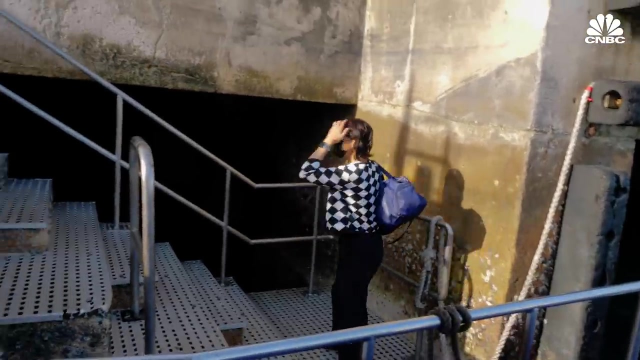 After the incineration process, my journey takes me on a ferry to the country's only landfill, located along the Singapore Strait, one of the busiest waterways in the world. I'm going to take a look at the landfill in the next few days. 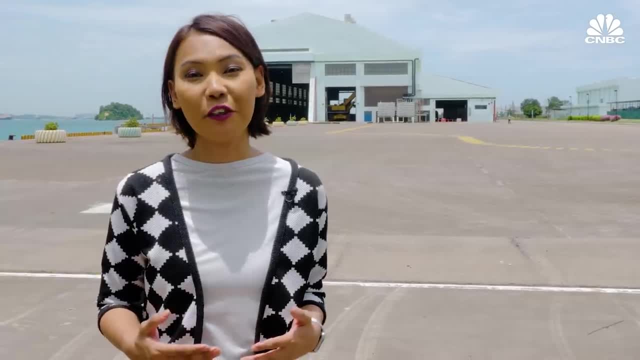 I'm going to take a look at the landfill in the next few days. I'm going to take a look at the landfill in the next few days. Semakau Landfill is an offshore landfill enclosed by a 4.3-mile perimeter rock embankment. 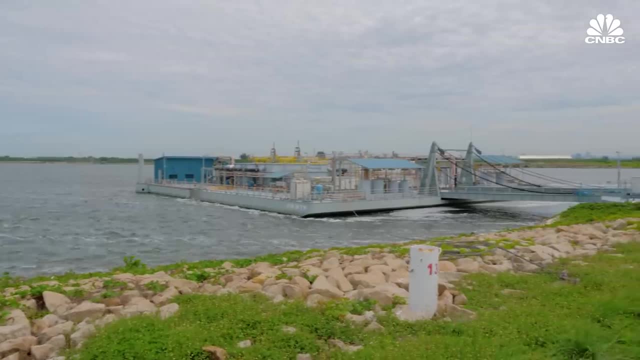 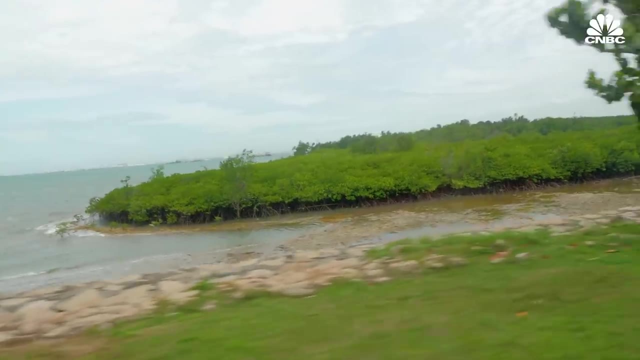 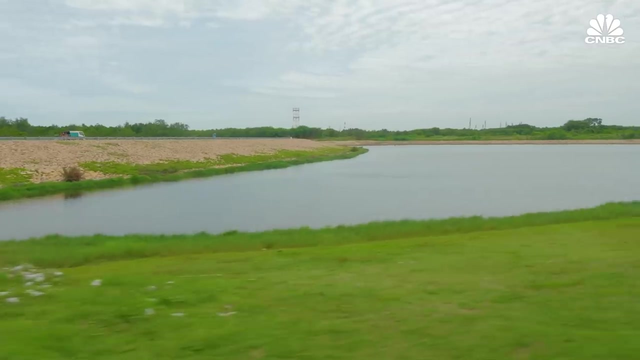 which creates a sea space to fill with incinerated rubbish, In operation since 1999 and costing nearly half a billion dollars. the island is more than just a landfill and costing nearly half a billion dollars. Actually, we make up of two big islands. 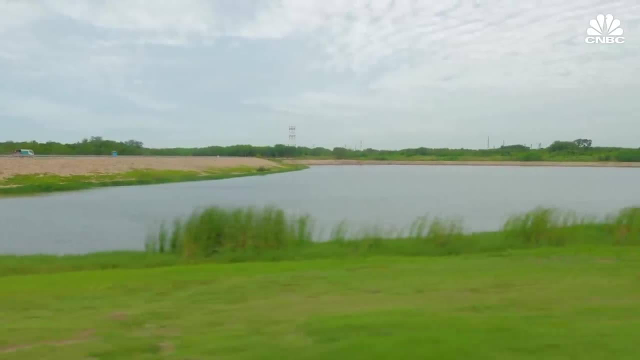 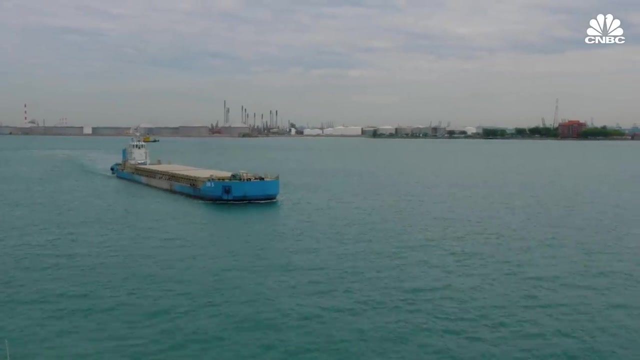 called the Pulau Semakau and Pulau Sake, And these are two joined together into what we call. what you see here: a 350 hectares Pulau Semakau landfill, A barge ferries, more than 2,000 tonnes of waste. 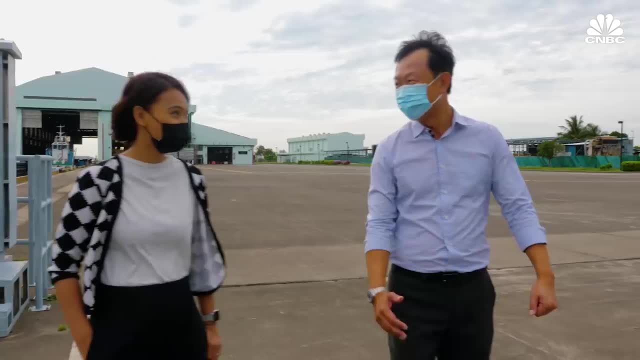 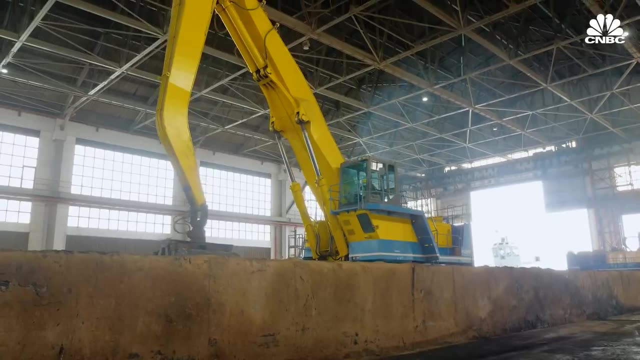 between mainland Singapore and Semakau Landfill daily, says Desmond Lee, General Manager of the landfill. We have big equipment such as the dump truck, excavators, etc. These are equipments that we use daily And you can hear. we have also the 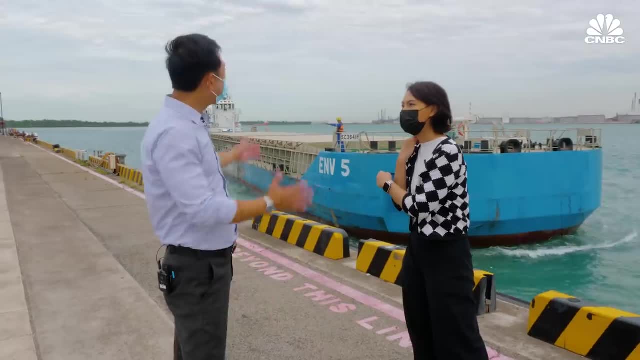 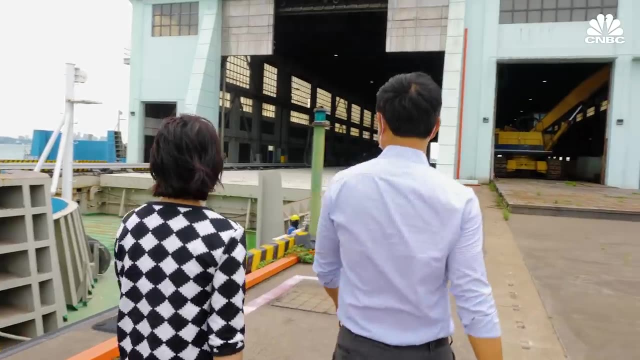 What's going on there? Yeah, These barges come from the Tuas Marine Transfer Station. From Tuas travel a 33-kilometre journey all the way here. Tell me about how the ash is going to get transferred out. 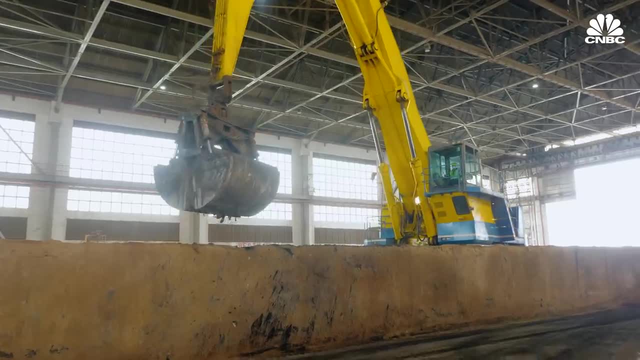 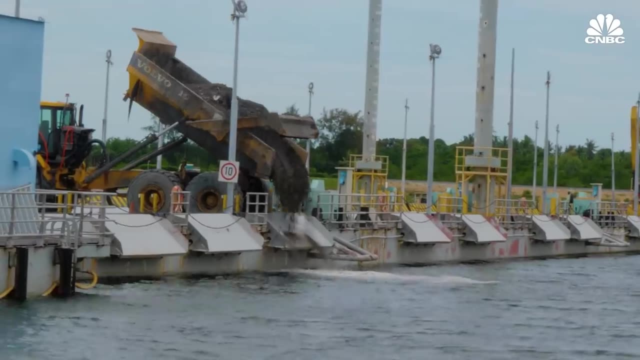 There is what you call the long-arm excavator. This excavator will grab the ash and the non-incinerated waste up and drop into what you call the dump truck. The trucks will then unload the ash into specific cells within the lagoon to prevent leaks and contamination of the seawater. 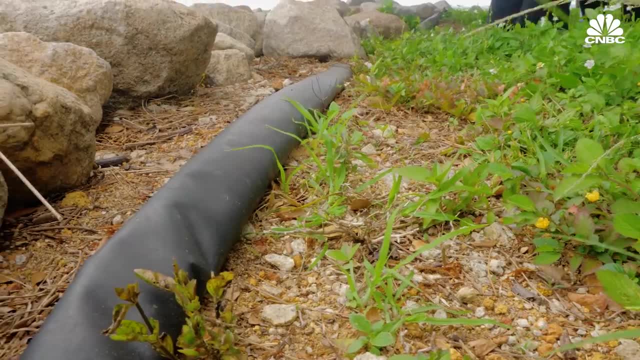 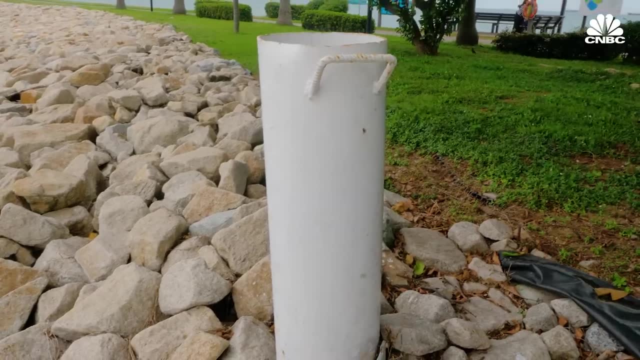 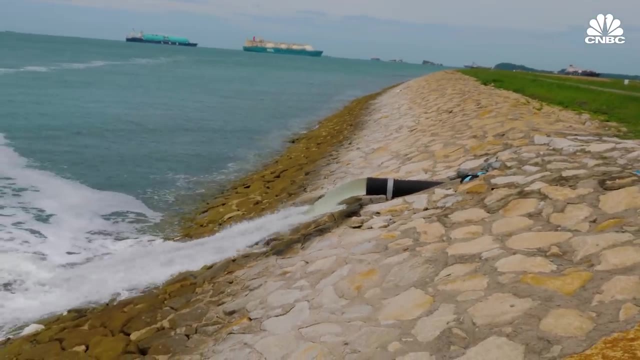 outside the rock buns, The perimeter is lined with impermeable membrane and a layer of marine clay. As the water level within the lagoon increases with rainfall and the dumping of the ash, the overflow is discharged into the open sea after being treated at a wastewater treatment plant. 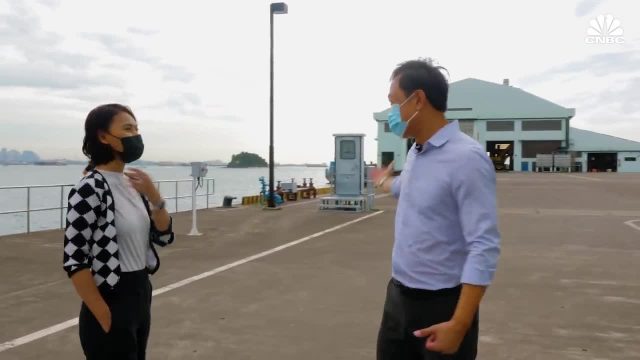 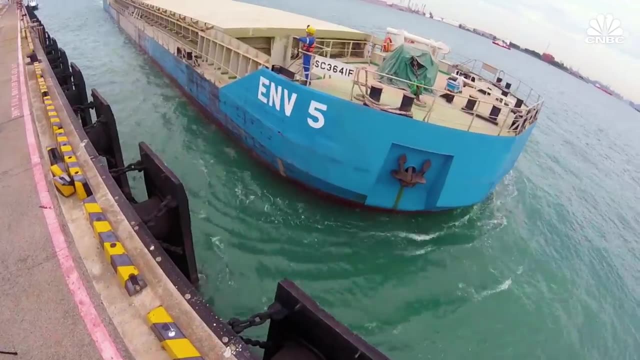 And you can hear. we have also the What's going on there. Yeah, These barges come from the Tuas Marine Transfer Station. From Tuas travel a 33-kilometre journey all the way here. Tell me about how the ash is going to get transferred out. 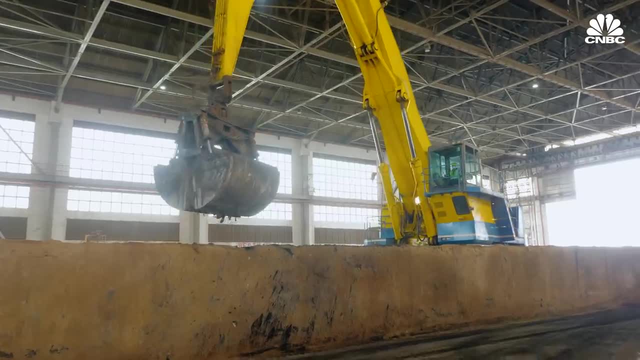 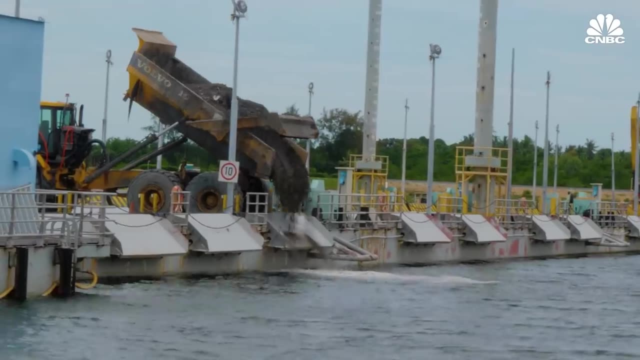 There is what you call the long-arm excavator. This excavator will grab the ash and the non-incinerated waste up and drop into what you call the dump truck. The trucks will then unload the ash into specific cells within the lagoon to prevent leaks and contamination of the seawater. 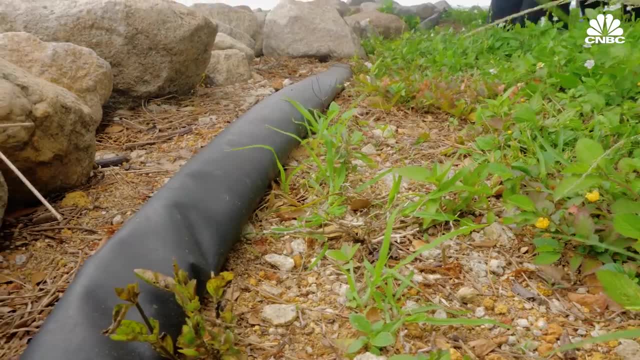 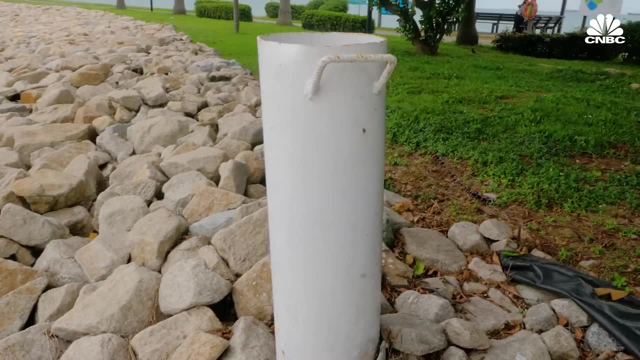 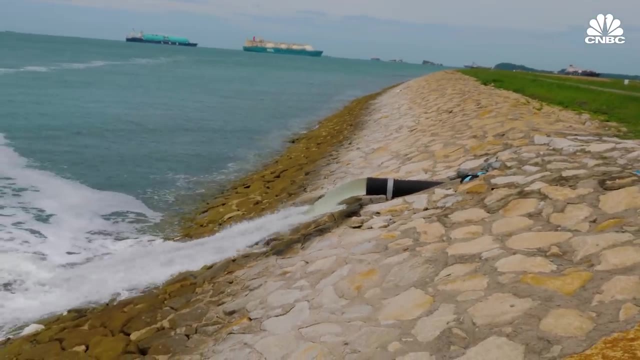 outside the rock buns, The perimeter is lined with impermeable membrane and a layer of marine clay. As the water level within the lagoon increases with rainfall and the dumping of the ash, the overflow is discharged into the open sea after being treated at a wastewater treatment plant. 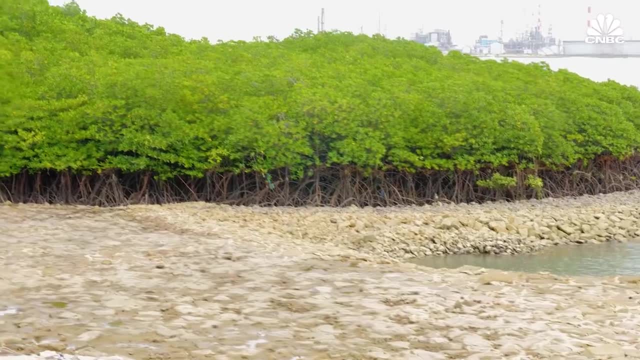 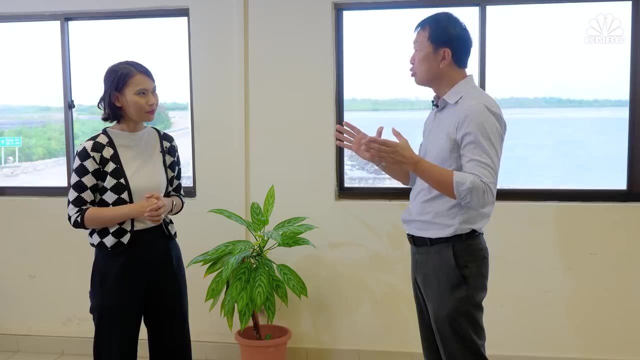 If you traverse around in Samakau, you will see there are a lot of mangroves around and there are also beautiful corals. This is a testimony to the absent or adverse impact from our operation in the landfill. We also want to ensure the marine life and nature. 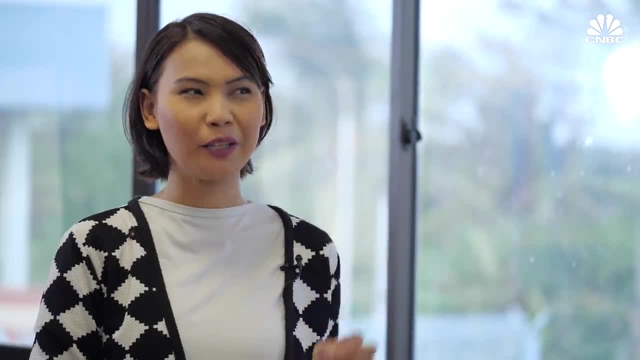 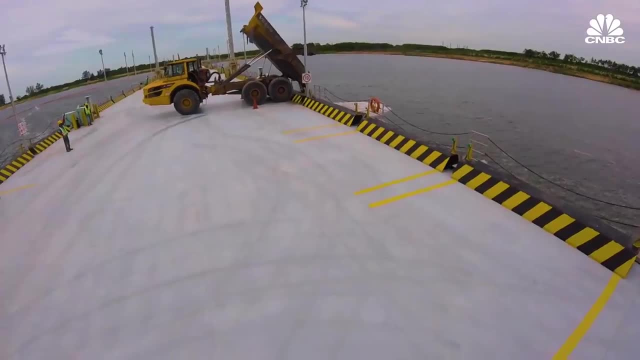 in this area continues to thrive. How filled is Samakau Landfill right now? Based on the current waste generation, Samakau Landfill will be completely filled by 2035.. However, there are current plans to work together with the different government agencies. businesses. 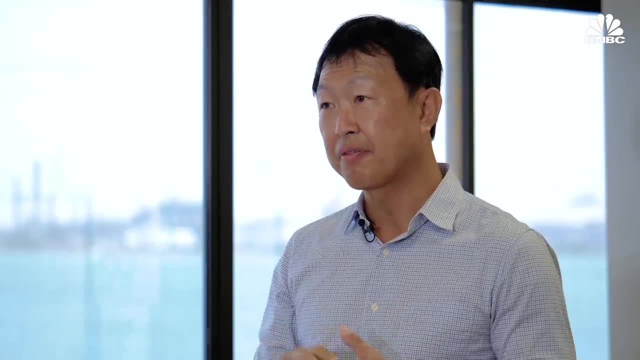 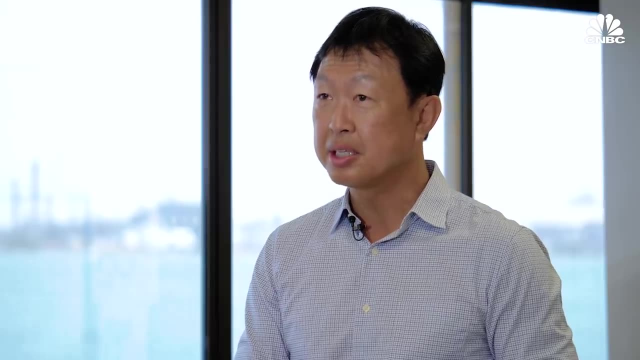 as well as the communities, to look into how we can extend the life of Samakau Landfill. What lessons can we learn from Singapore's other previous landfills? One key lesson that we learned is that it takes a long time to remediate the landfill. 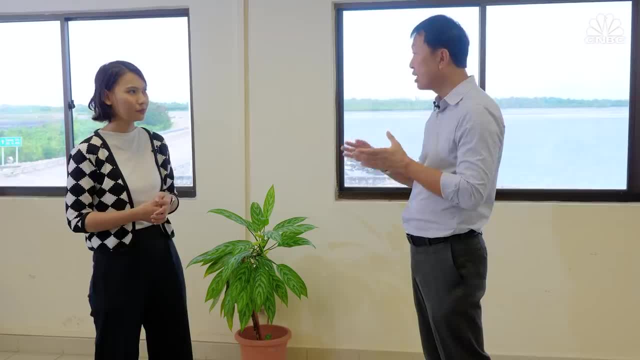 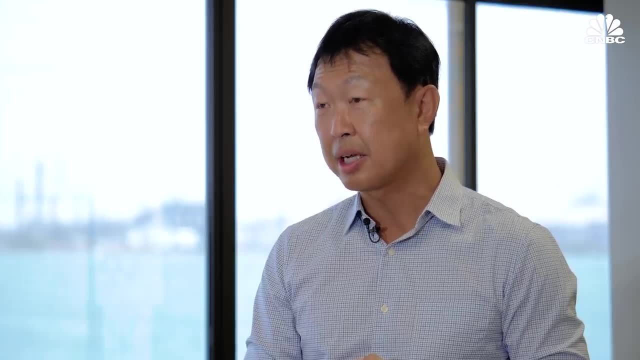 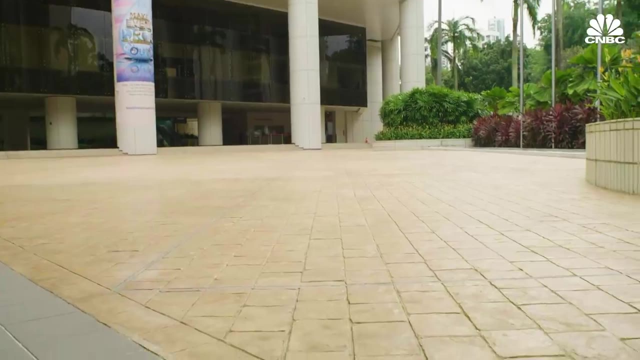 and then there's also resources need to be committed to them before the land can be remediated for other uses. The other strategy we are also taking is looking at the possibilities of recycling the insulation bottom ash, which is now known as new sand and could be used for non-structural concrete, for example. 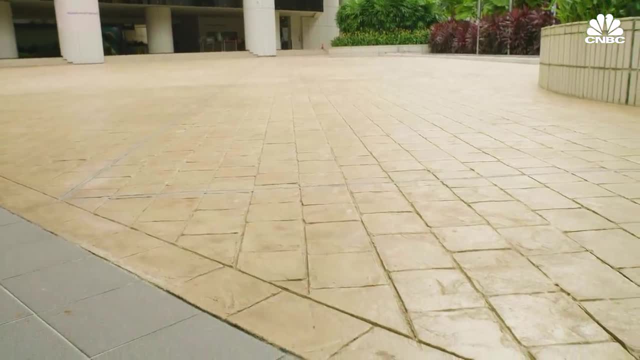 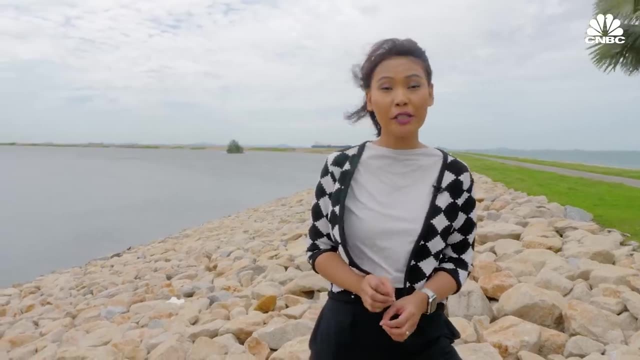 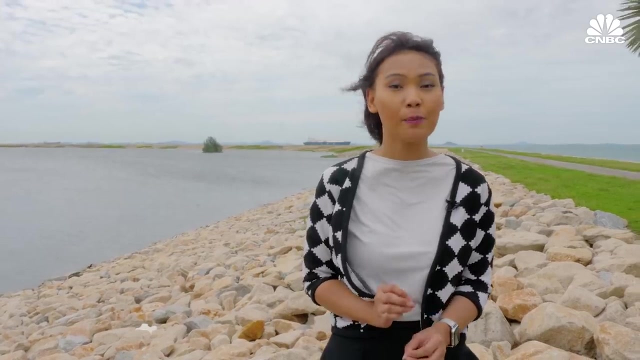 To date, new sand has been used to create footpaths and benches, which are ongoing for its application in road construction projects. Landfills are a short-term solution to a long-term problem In land-scarce Singapore, which is slightly smaller than New York City. 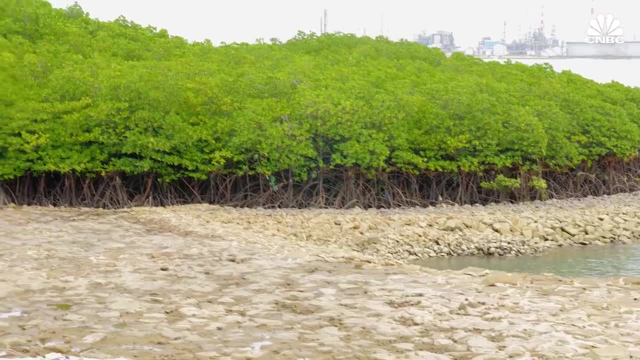 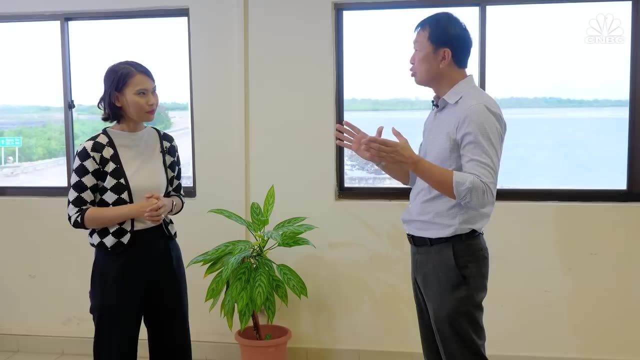 If you traverse around Semakau, you will see there are a lot of mangroves around and there are also beautiful corals. This is a testimony to the absent or adverse impact from our operation in the landfill. We also want to ensure the marine life and nature. 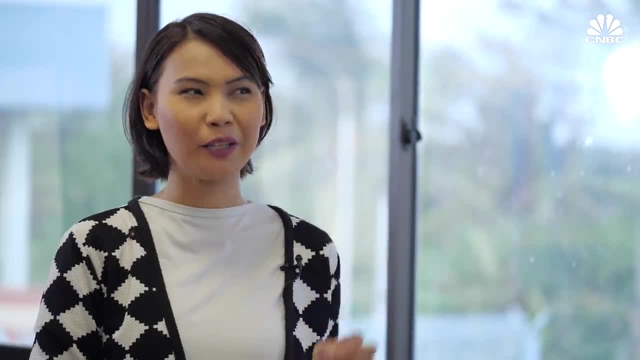 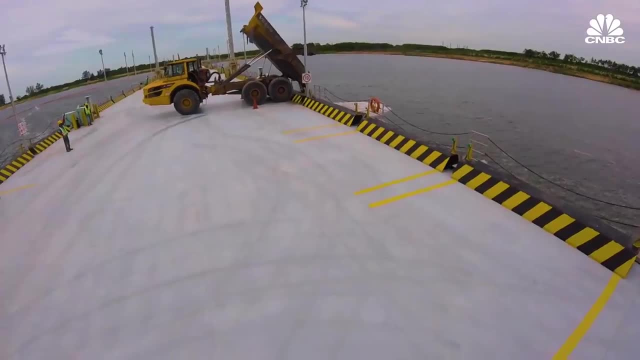 in this area continues to thrive. How filled is Semakau Landfill right now? Based on the current waste generation, Semakau Landfill will be completely filled by 2035.. However, there are current plans to work together with the different government agencies. businesses. 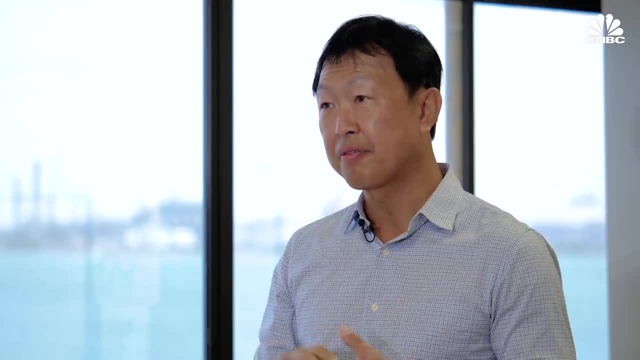 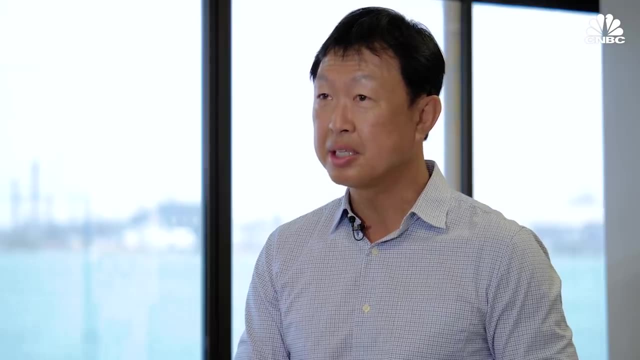 as well as the communities, to look into how we can extend the life of Semakau Landfill. What lessons can we learn from Singapore's other previous landfills? One key lesson that we learned is that it takes a long time to remediate the landfill. 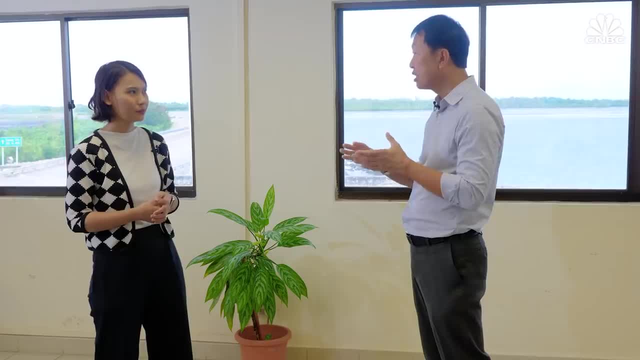 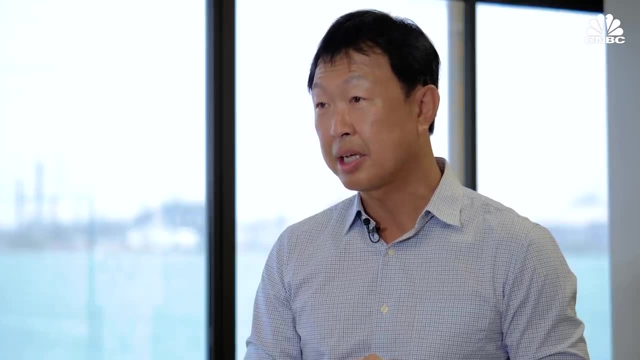 and then there are also resources that need to be committed to them before the land can be remediated for other uses. The other strategy we are also taking is looking at the possibilities of recycling the insulation bottom ash, which is now known as new sand and could be used for non-structural concrete, for example. 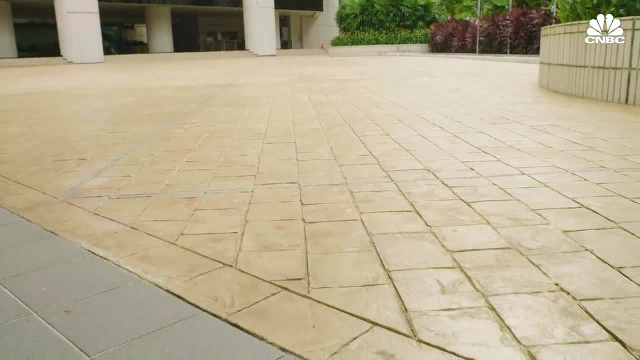 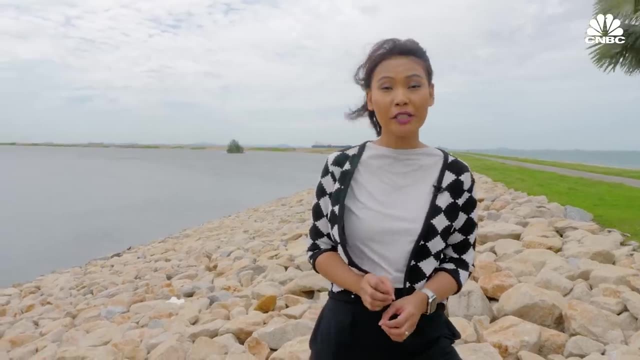 To date, new sand has been used to create footpaths and benches and is ongoing for its application in road construction projects. Landfills are a short-term solution to a long-term problem In land-scarce Singapore, which is slightly smaller than New York City. 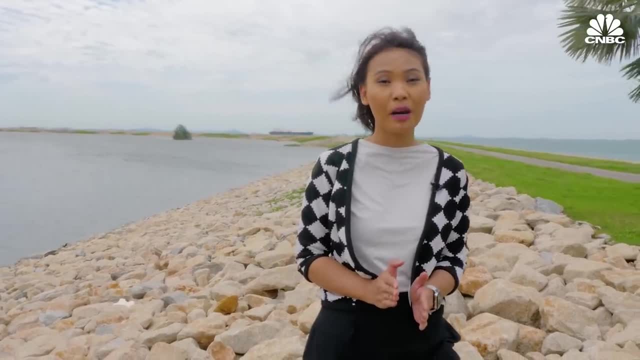 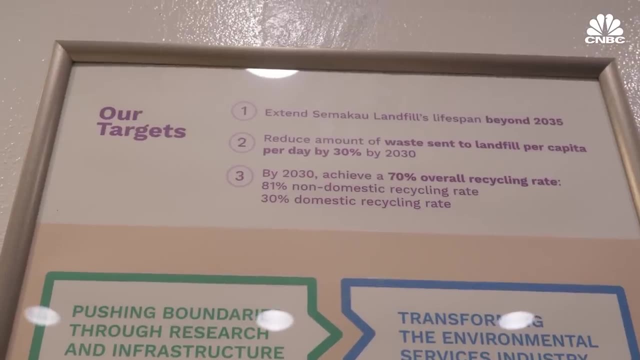 space is a luxury and it's a matter of time before Semakau Landfill is full. Singapore aims to reduce the waste going into Semakau Landfill by 30% by 2030 as part of its Zero Waste Master Plan. The country also intends to develop new ways of recycling waste. 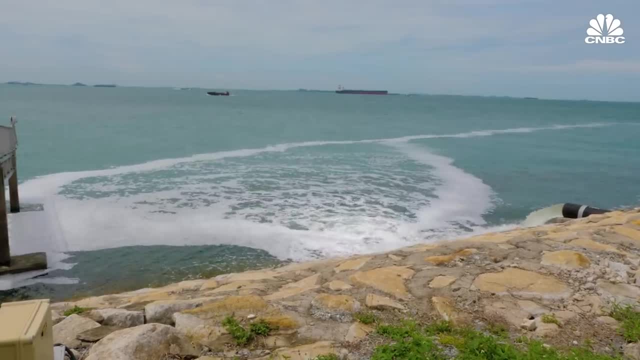 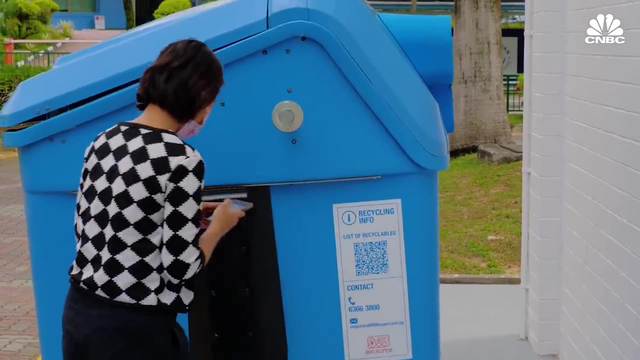 The country also intends to develop new ways of recycling waste. The country also intends to develop new ways of recycling waste to meet the treatment needs of waste, water, sludge and even food waste, ultimately improving the recycling rate in Singapore, Despite the high rates of recycling among developed nations. 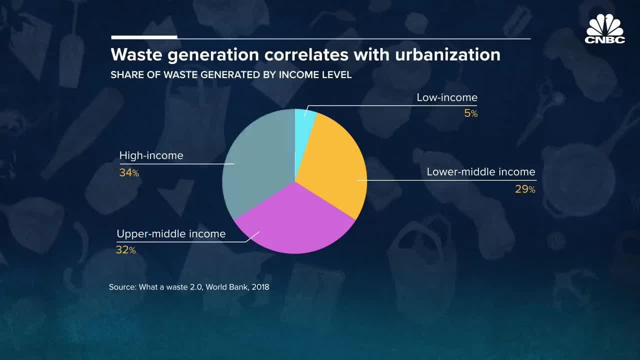 high-income countries, which account for 16% of the world's population, generate 34% of global waste. Conversely, about 5% of the world's waste come from low-income countries, even though they make up 9% of the world's population. 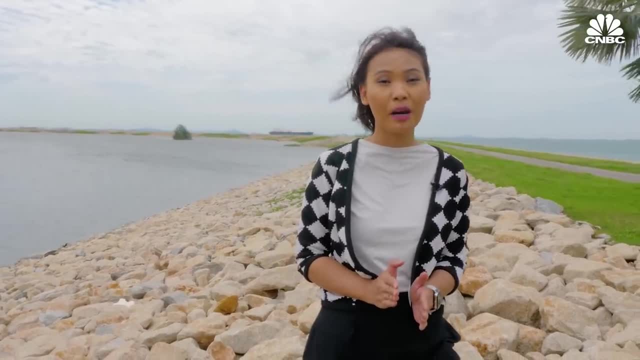 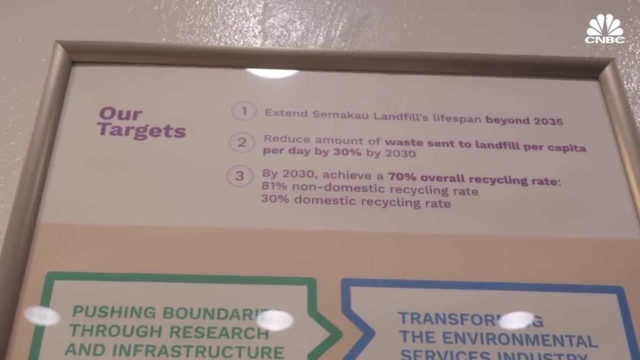 space is a luxury and it's a matter of time before Samakau Landfill is full. Singapore aims to reduce the waste going into Samakau Landfill by 30% by 2030 as part of its Zero Waste Master Plan. 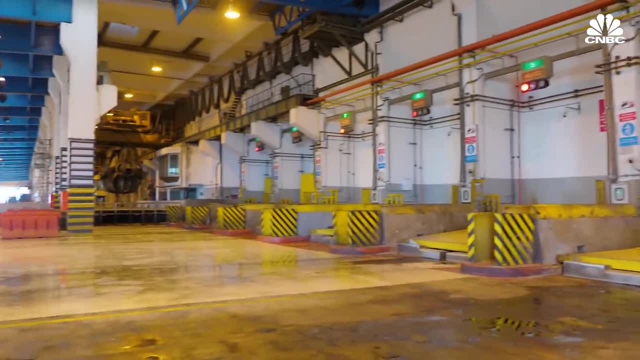 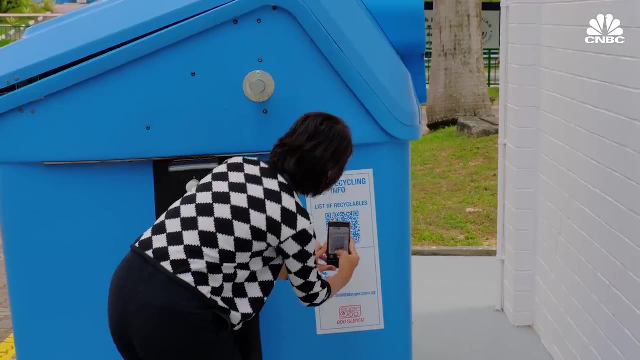 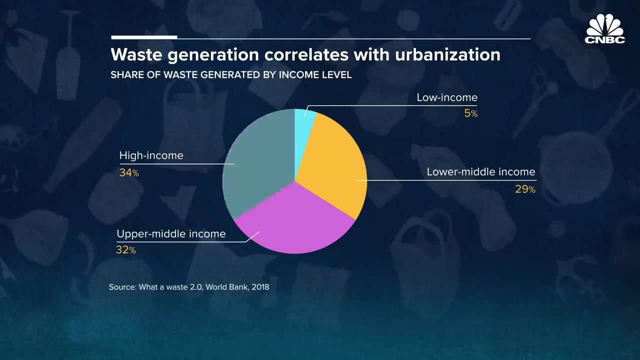 The country also intends to develop new waste management facilities to meet the treatment needs of wastewater sludge and even food waste, ultimately improving the recycling rate in Singapore, Despite the high rates of recycling among developed nations, high-income countries, which account for 16% of the world's population. 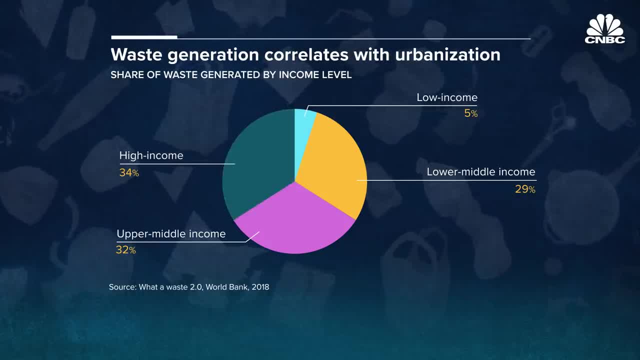 generate 34% of global waste. Conversely, about 5% of the world's waste come from low-income countries, even though they make up 9% of the world's waste. The US, Canada and Bermuda- all high-income countries in North America. 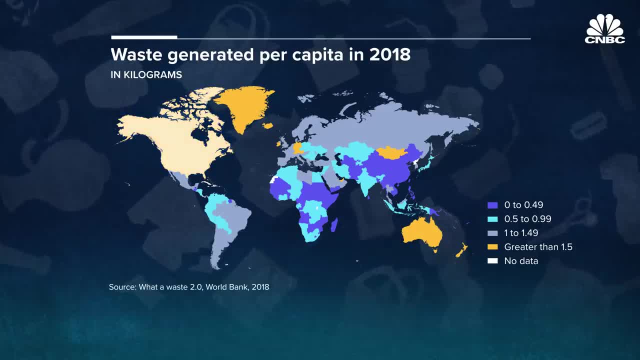 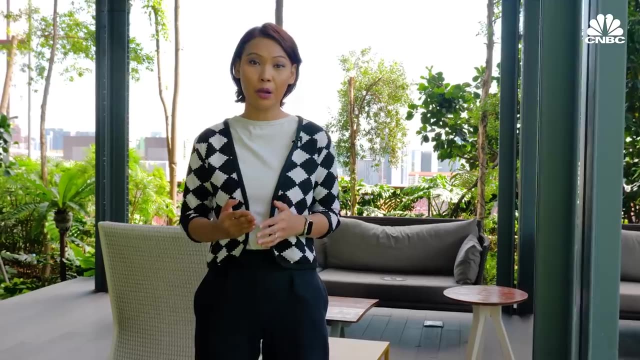 generate one of the highest average amount of waste per capita. However, the trend is expected to reverse in the next few decades, as low-income countries experience economic growth and a population boom. For over two decades, China was the dumping ground for nearly half of the world's scrap. 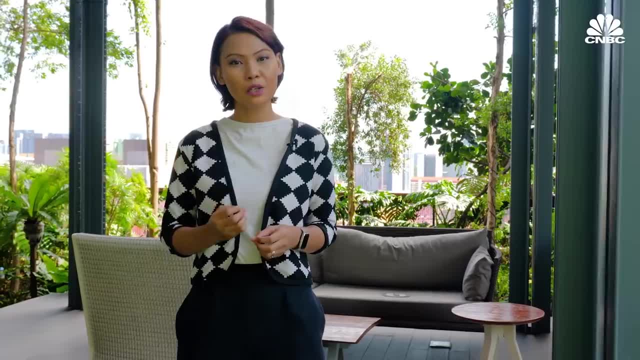 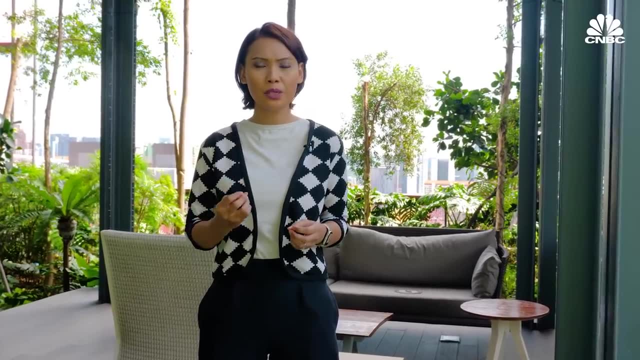 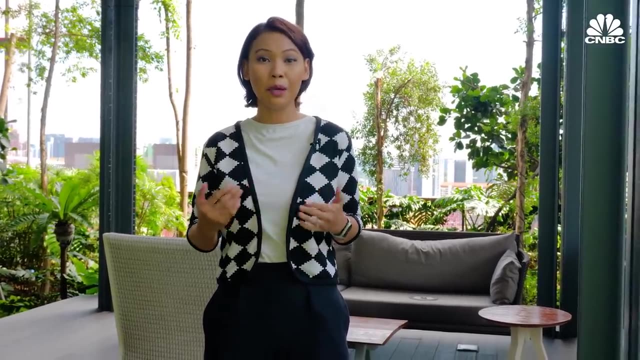 with much of it originating from developed countries such as the United States, The US, UK and Australia. All that changed in 2018, when China imposed a blanket ban on 24 types of imported waste, citing the need to protect its environment and public health. 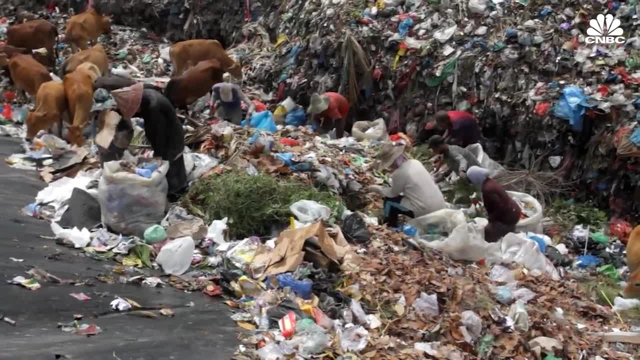 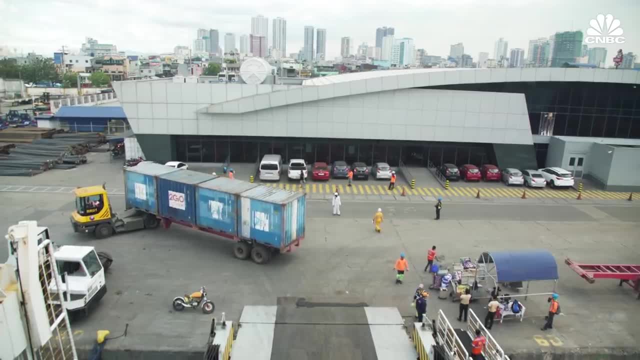 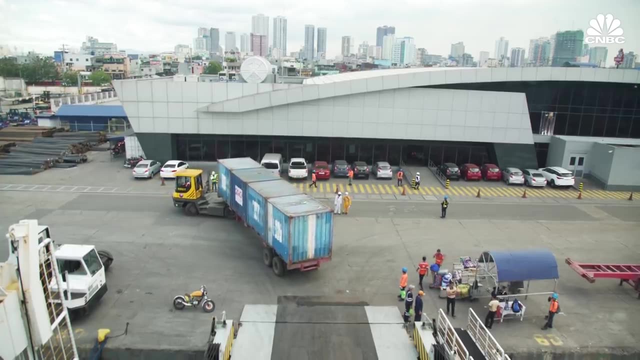 The magnitude of the problem was laid bare when other countries in Southeast Asia also started rejecting plastic waste from the rich industrialized countries. In 2019, the Philippines sent back containers of waste to Canada and South Korea, while waste from Spain and Australia that were sent to Malaysia was similarly rejected. 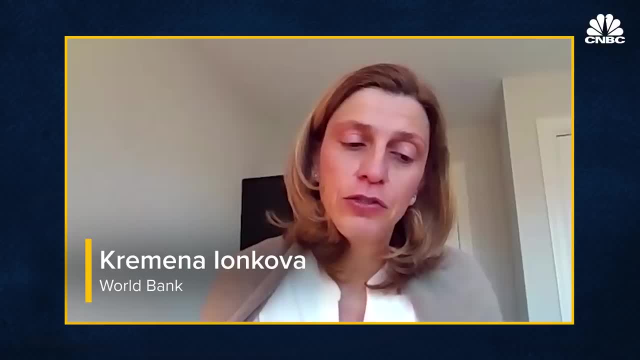 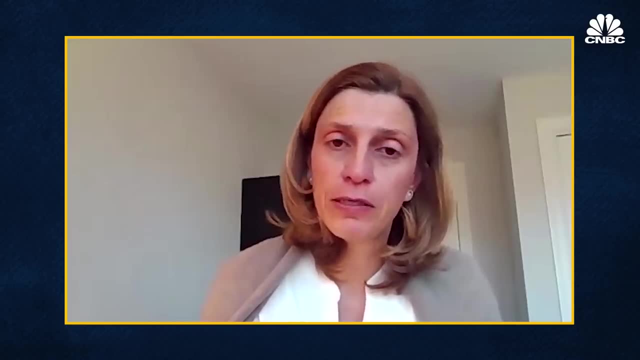 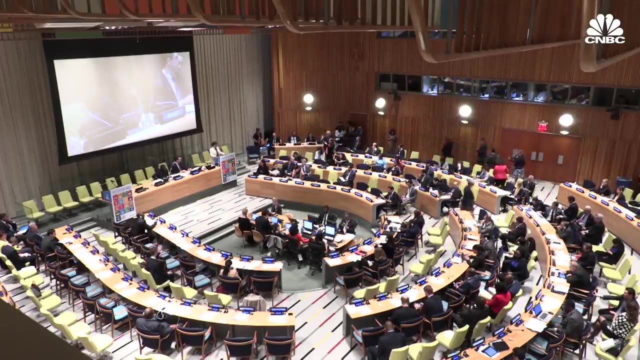 Waste management is very expensive And it should not be looked at as being an economic activity to generate revenue, but as a public service that requires financing, Not just financing that is affordable for the population and for the country as such, but also in terms of legislative environment and regulation. 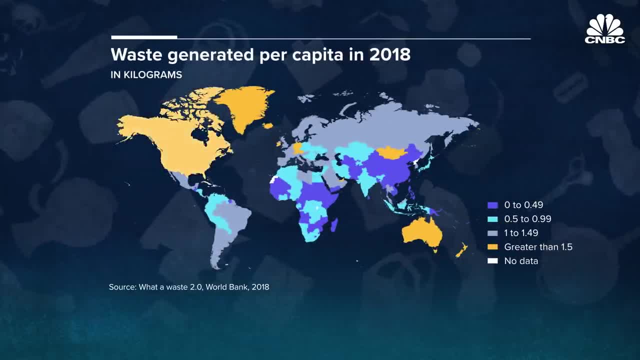 even though they make up 9% of the world's population. even though they make up 9% of the world's population, Notably the US, Canada and Bermuda- all high-income countries in North America- generate one of the highest average amount of waste per capita. 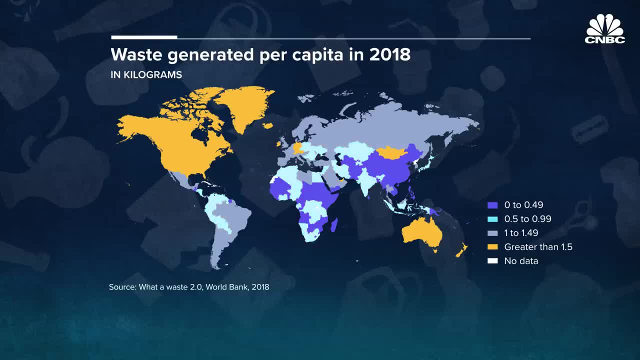 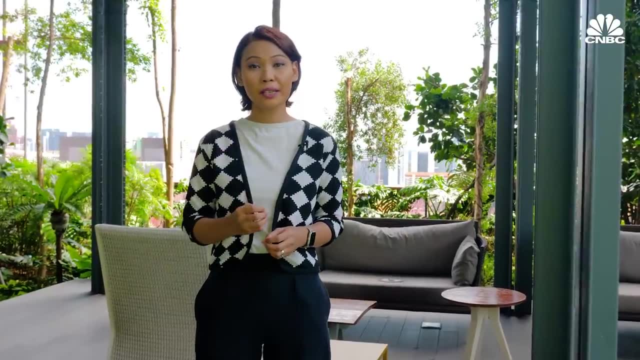 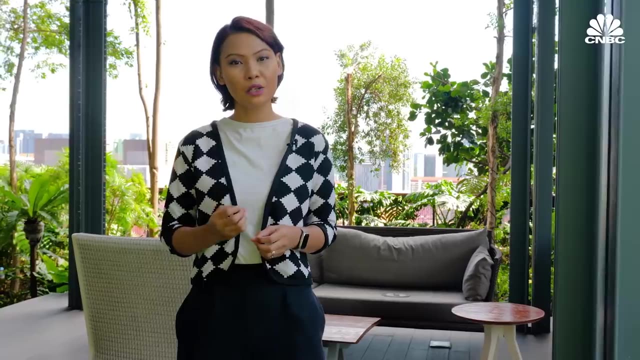 However, the trend is expected to reverse in the next few decades, as low-income countries experience economic growth and a population boom. For over two decades, China was the dumping ground for nearly half of the world's scrap, with much of it originating from developed countries. 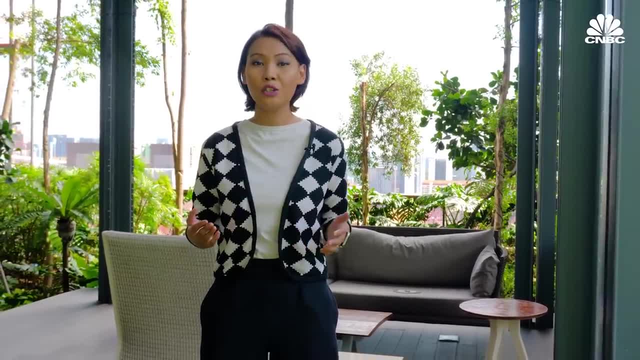 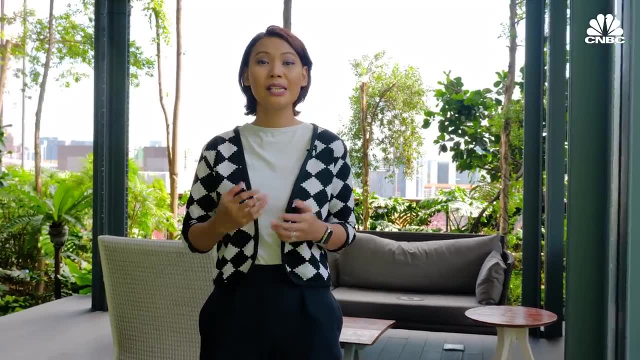 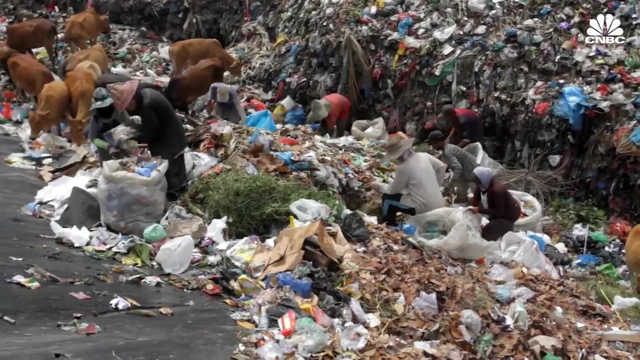 such as the US, UK and Australia. All that changed in 2018, when China imposed a blanket ban on 24 types of imported waste, citing the need to protect its environment and public health. The magnitude of the problem was laid bare when other countries in Southeast Asia 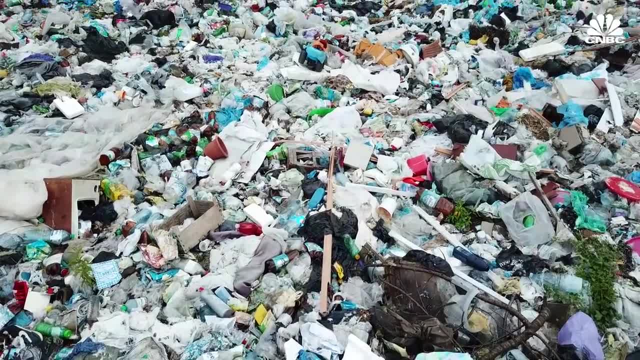 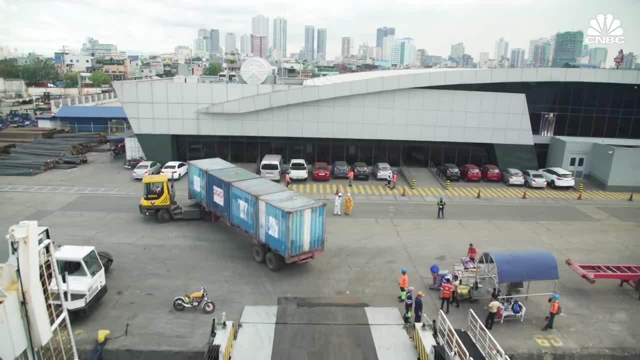 also started rejecting plastic waste from the rich industrialized countries. In 2019,, the Philippines sent back containers of waste to Canada and South Korea. In 2019, the Philippines sent back containers of waste to Canada and South Korea, while waste from Spain and Australia that were sent to Malaysia was similarly rejected. 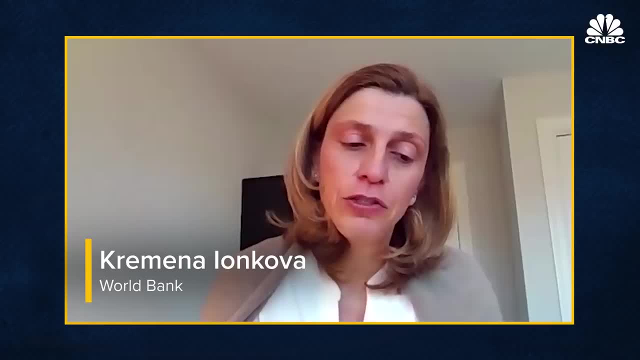 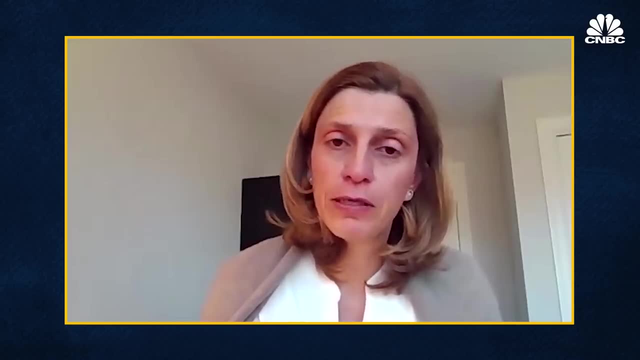 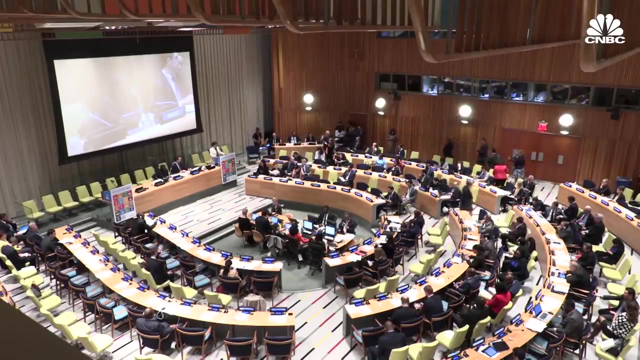 Waste management is very expensive And it should not be looked at as being an economic activity to generate revenue, but as a public service that requires financing, Not just financing that is affordable for the population and for the country as such, but also in terms of legislative environment. 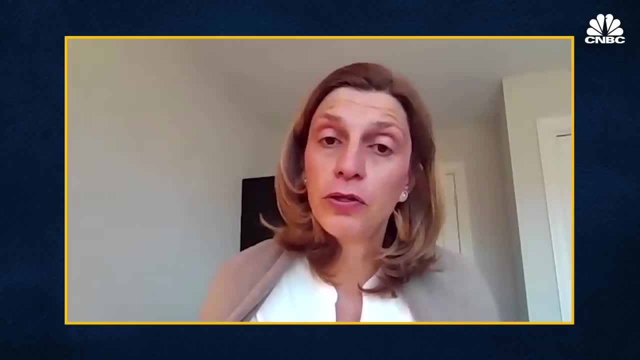 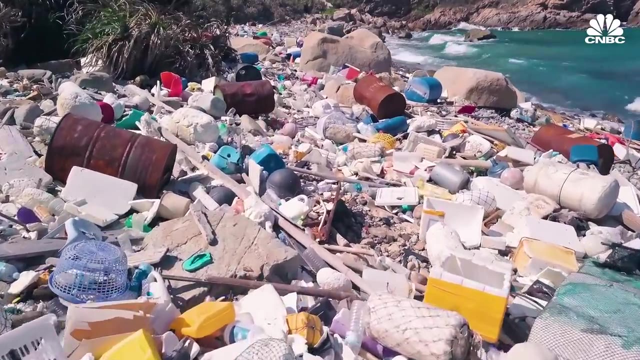 and regulation, and monitoring and enforcement. All of these pieces of the puzzle should be in place because, at the end of the day, as we have seen many times, there is always an easy way out, and that is to pollute the environment. 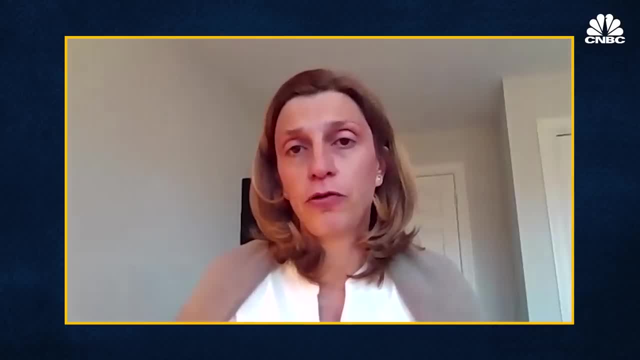 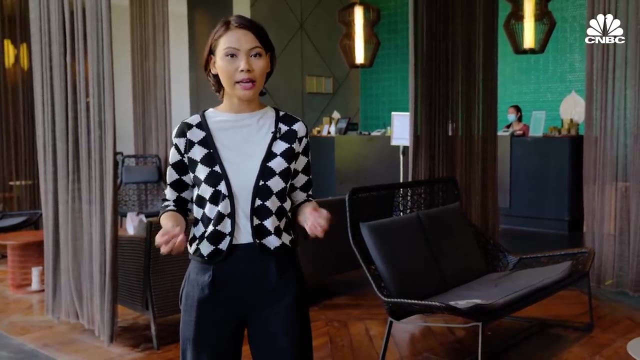 It takes years and concerted effort to switch the way we as a society behave so that we increase. It takes years and concerted effort to switch the way we as a society behave so that we increase. More companies are also applying environmental, social 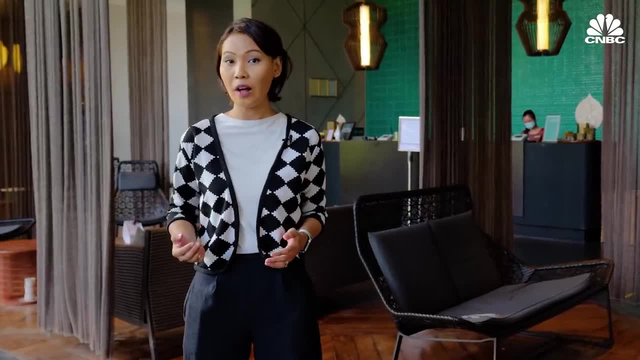 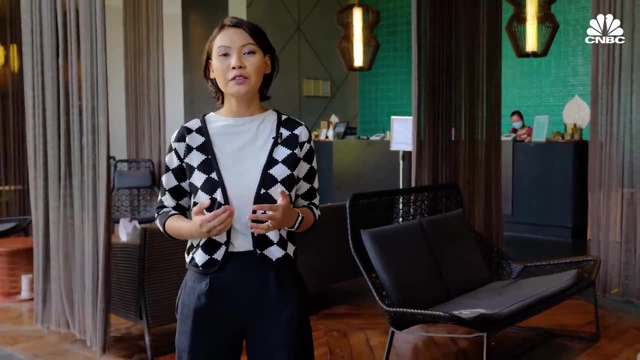 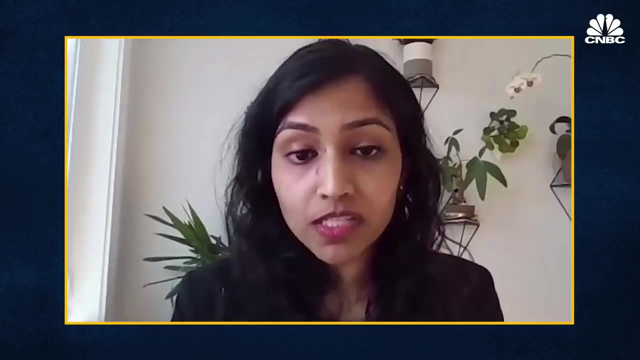 and corporate governance standards to their operations. While this is the latest trend in town, it remains to be seen if businesses can be both ethical and profitable, benefiting stakeholders, society and the planet. Citizens are key to changing the waste management system moving forward.